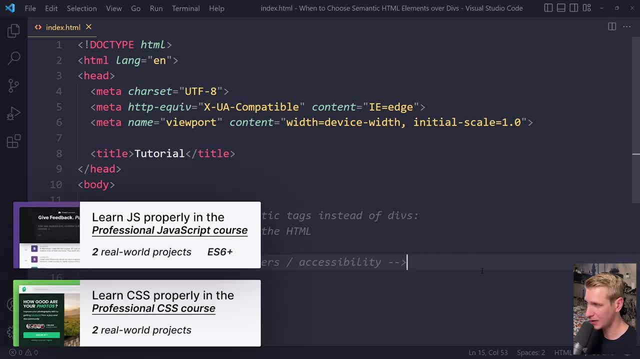 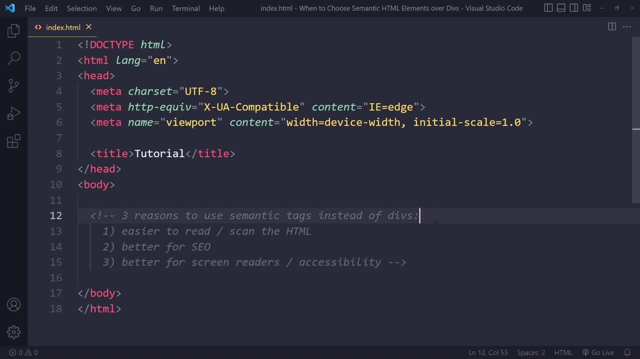 In this tutorial, we'll discuss why and when to use semantic HTML elements over divs. All right, so I just have a couple of examples for you. But first of all, why do we even want to use semantic tags instead of divs? Well, first of all, it's easier to read and scan the HTML if 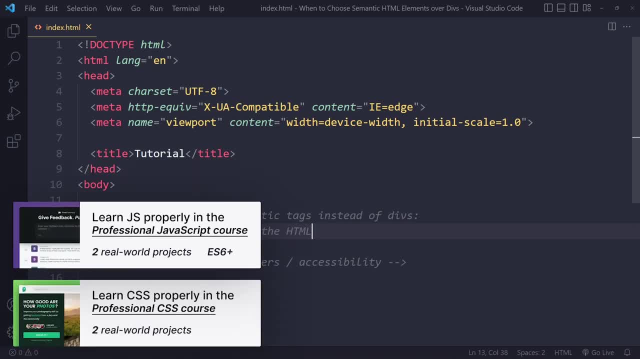 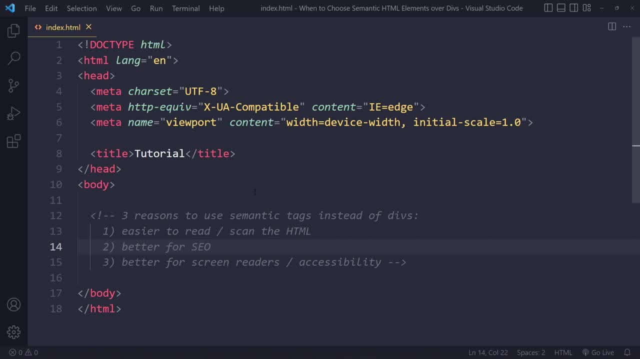 it has been properly structured with these semantic tags, and I'll show you why in a second. It's also better for SEO. It makes it easier for those search engines like Google to come to your website and properly index all the content that's on there, which in turn will 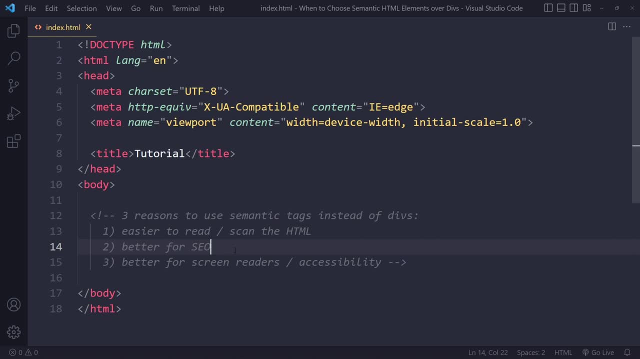 make it more likely that you rank higher in their search engine results. right, so you get more traffic. And it's also better for screen readers or assistive technology to properly, you know, categorize and index what's going on on your website. So that's also better for accessibility. 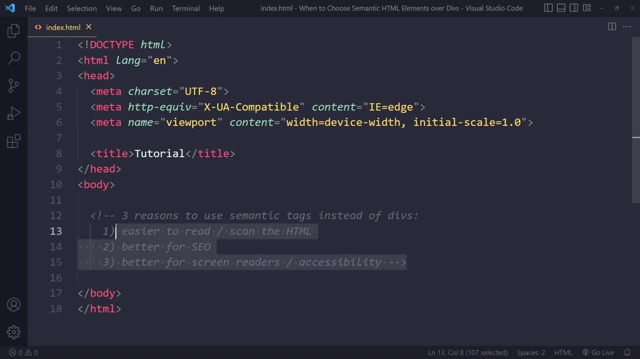 These are the three main reasons for why we want to use semantic tags. So let me actually just give you an example of what a very typical HTML boilerplate would look like. So this is currently basically an empty HTML file. Now, globally speaking, you're going to have a header- usually. 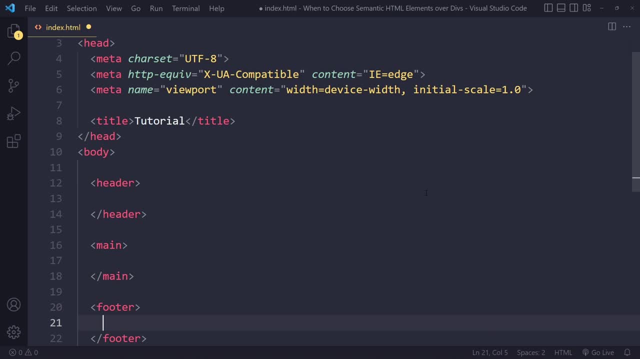 a main section and a footer section, And so these are already semantic tags, because you could also use divs right. You could use divs. Div stands for divider right. You could use that. Practically they would work the same, But in practice, if you want to use semantic tags, 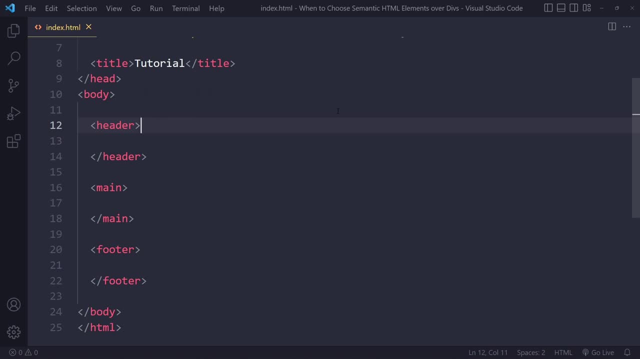 this is what you're going to get. So header is usually for introductory content. you know, like the logo, like the introductory links, The main is really for the dominant content on the page and the footer is for, you know, maybe some other links like terms. 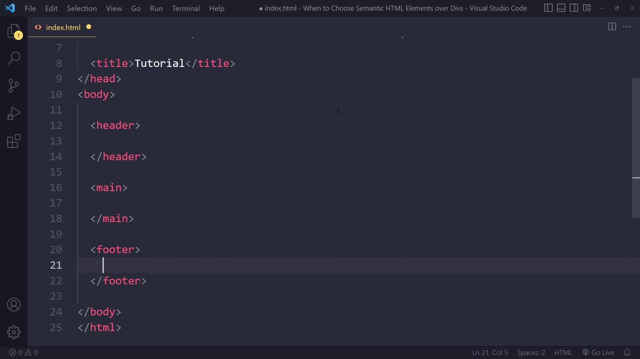 and definitions, privacy policy- not really important stuff going on there. So in the header then typically you also have some kind of nav. So the nav is really for the most important links on the page or like the most important navigation on the page. Typically people structure it like this: 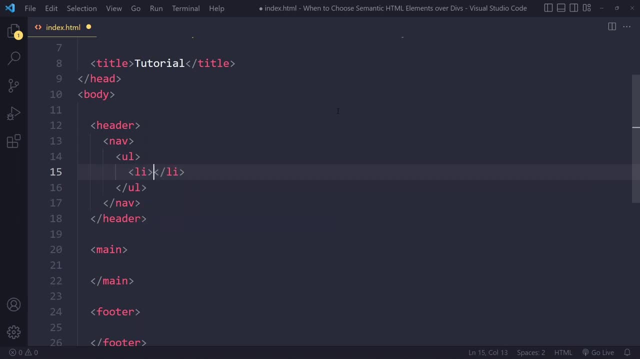 So you're going to have a list of links. So in a list we have LIs, So it's going to be quite nested here, And then in here you're going to have the actual anchor tag, And so usually you're going. 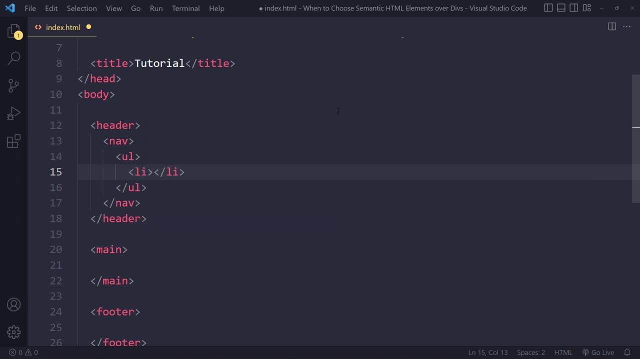 so you're going to have a list of links. So in a list we have LIs that's going to be quite nested here, And then in here you're going to have the actual anchor tag. Usually you're going to have a. 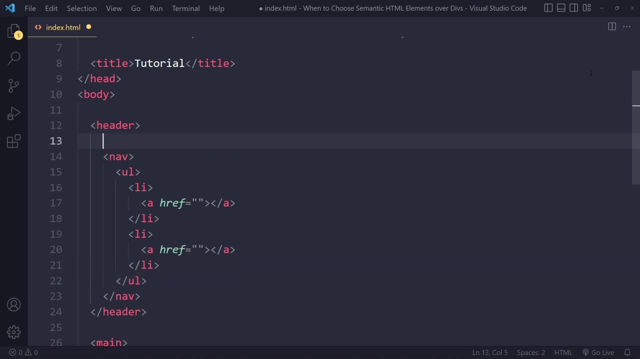 bunch of links here also have like a logo right the logo that could be just an image, let's say right, so you would have an image in the in the header, and then you would have a nav right. so it's quite nested here. but this would be a pretty typical semantic structure in the header. then in the main, the dominant. 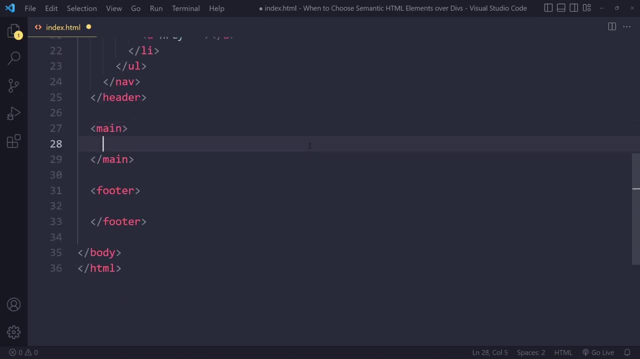 content on the page. usually you're going to have a bunch of sections, as it's called, right. so in practice a lot of people would use div, but it's better to use section, and i'll show you some practical examples on real world access websites in a second. but usually the main consists of a. 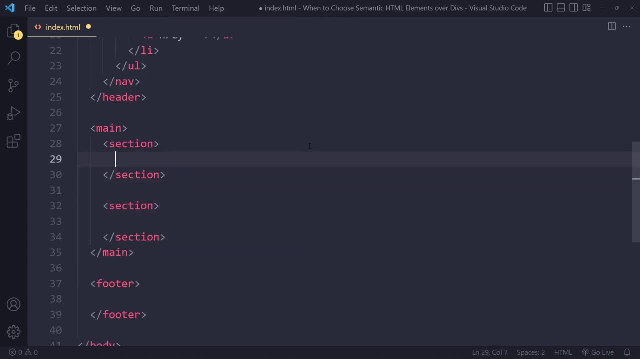 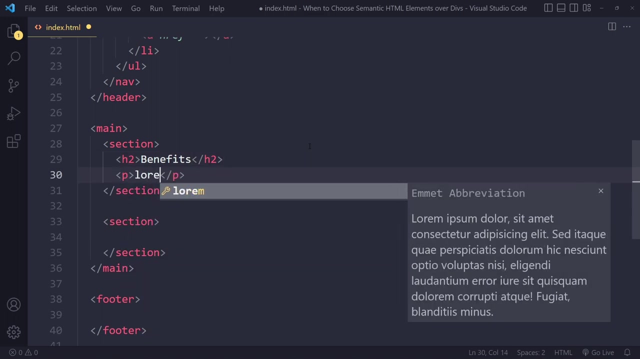 bunch of sections right, and then in the section you can have a heading right, so maybe an h1 or h2, and you would say something like: about us, maybe, or maybe some kind of a benefit section- let's do that, it's a bit more realistic- and then perhaps a paragraph section with a bunch of words. 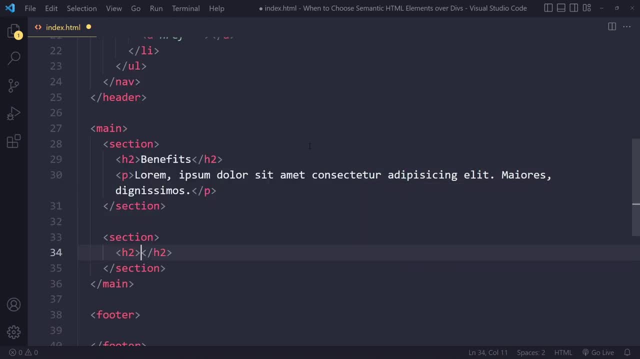 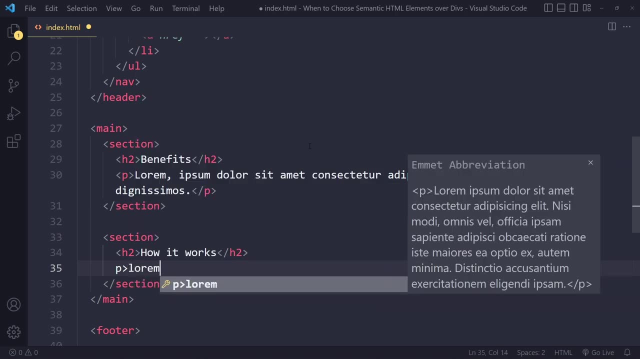 and that would be a section. and then you would have another section: benefits instead of benefits. we would have something like: um, how it works, right, and maybe some paragraph with a bunch of text. so in practice, what you see a lot of people do is they use div here, but it's better to use section. 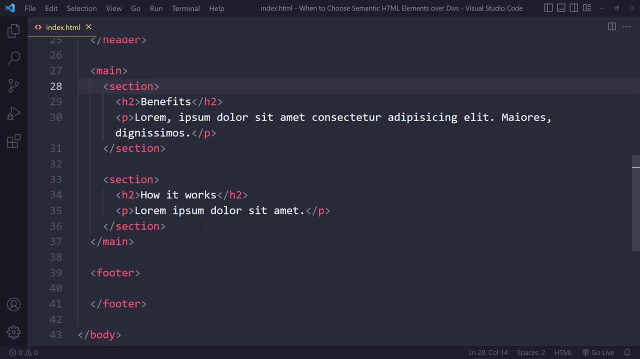 so why section instead of div? um? i'll show you that in a second on real world extras, uh websites, um. but in practice, what you also have in the main sometimes is have some kind of sidebar or some related content. that's not really the not really uh, something that should get the focus. 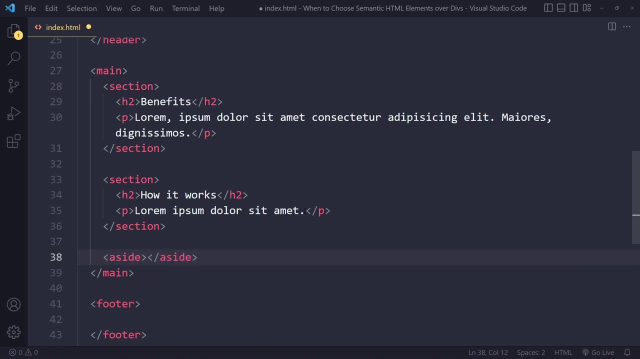 but you could have something like an aside in here as well. that's also what you see. sometimes this could be for a sidebar or something like that. you're also going to see the article tag. sometimes it's a bit trickier. this one, this one, is more suitable for if you can pull out. 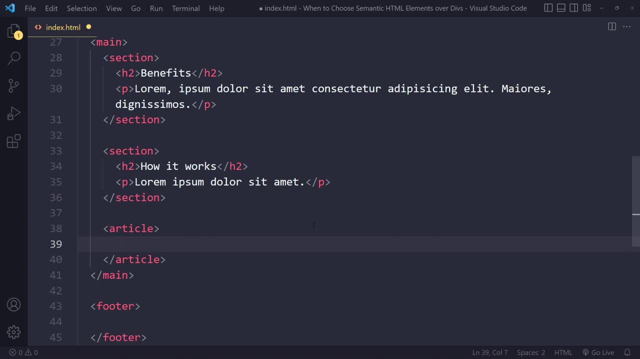 this content and place it somewhere else, and it wouldn't lose any meaning, right? so this is a bit more um, rare, and then in the footer usually um, you know you're gonna have a bunch of links, maybe some text, but here you would also use that nested structure again, except 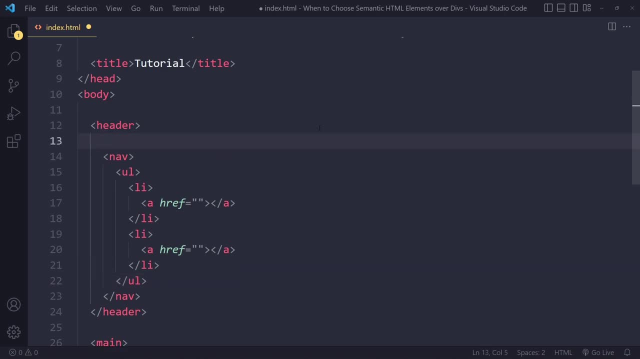 to have a bunch of links here, also have like a logo right. the logo that could be just an image, let's say right, so you would have an image in the in the header, and then you would have a nav right. so it's quite nested here. but 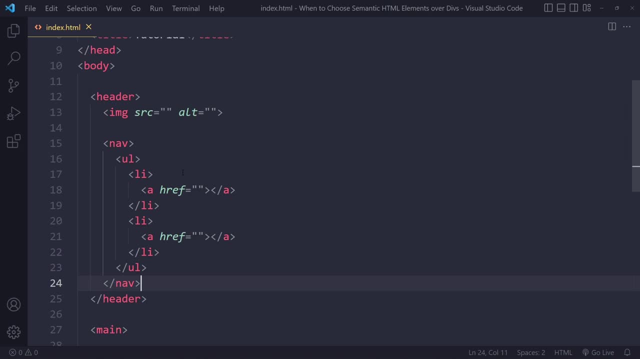 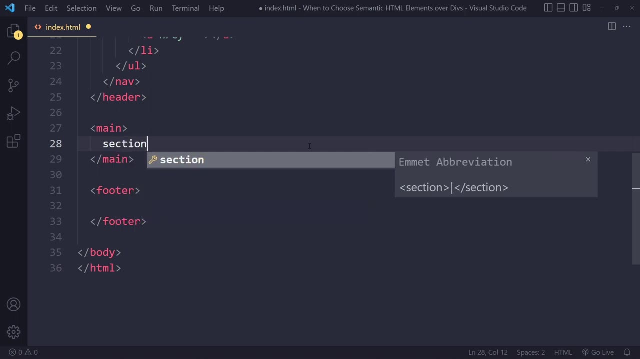 this would be a pretty typical semantic structure in the header, then in the main, the dominant content on the page. usually you're going to have a bunch of sections, as it's called, right. so in practice a lot of people would use div. but it's better to use section and i'll show you some. 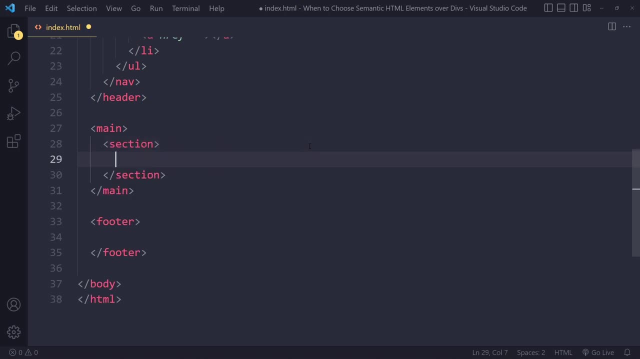 practical examples on real world access websites in a second. but usually the main consists of a bunch of sections right and then in the section you can have a heading right, so maybe an h1 or h2, and you would say something like: about us maybe, or maybe some kind of a benefit section. 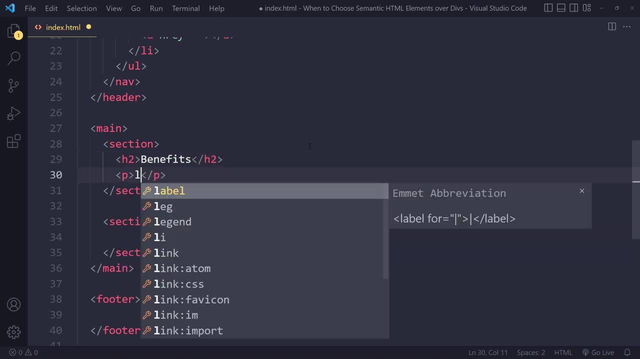 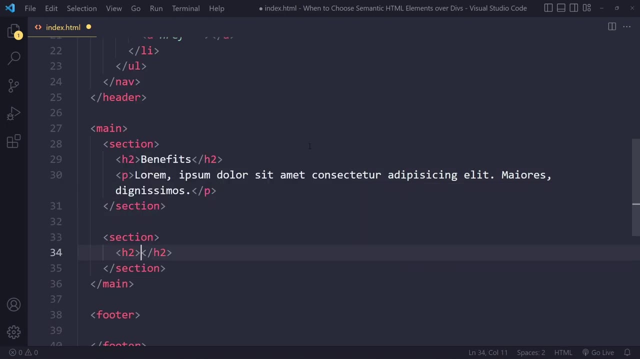 let's do that. it's a bit more realistic- and then perhaps a paragraph section with a bunch of words and that would be a section, and then you would have another section: benefits. instead of benefits. we would have something like: um, how it works right, and maybe some paragraph with a bunch of text. 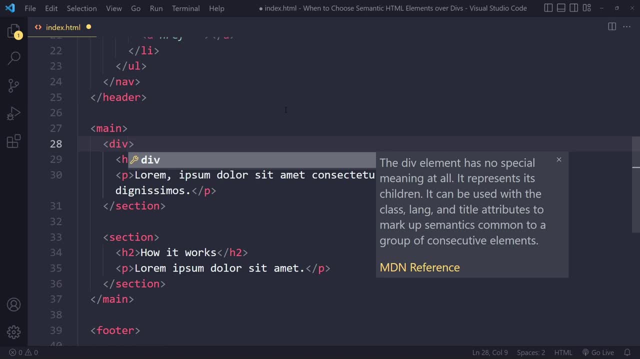 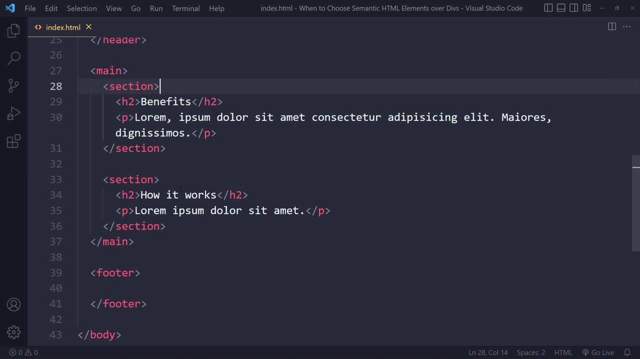 so in practice, what you see a lot of people do is they use div here, but it's better to use section. so why section instead of div? um? i'll show you that in a second on real world extras, uh websites um. but in practice, what you also have in the main sometimes is have some kind of sidebar. 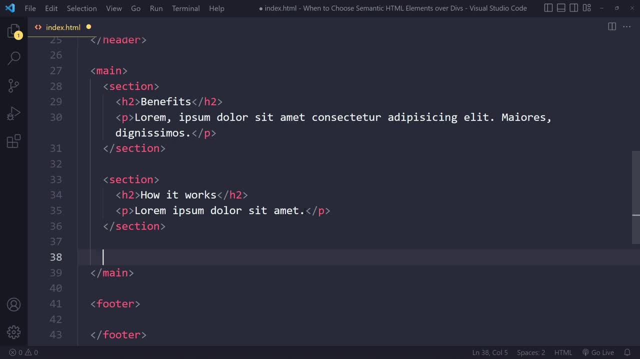 or some related content. that's not really the not really uh, something that should get the focus. but you could have something like an aside in here as well. that's also what you see sometimes. this could be for a sidebar or something like that. you're also going to see the article tag sometimes. 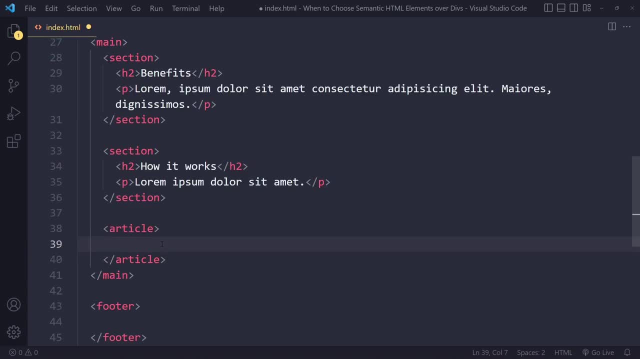 it's a bit trickier. this one, this one is more suitable for if you can pull out this content and place it somewhere else and it wouldn't lose any meaning, right? so this is a bit more rare. and then in the footer usually you know you're going to have a bunch of links maybe. some text. but here you would also use that nested structure again, except now you're going to want to place it. but again, you won't see a lot of fire in these, but we're going to focus on the out of these. that nested structure again, except now you're going to want to take out the images again and drawing. 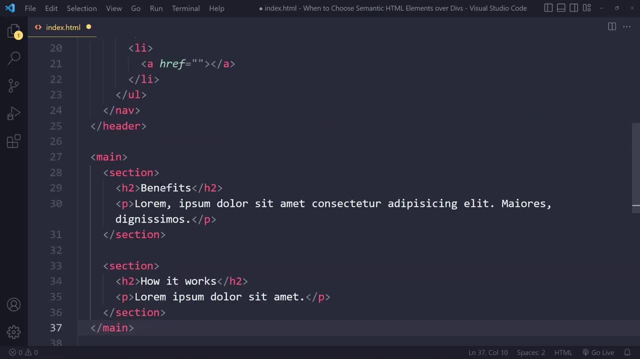 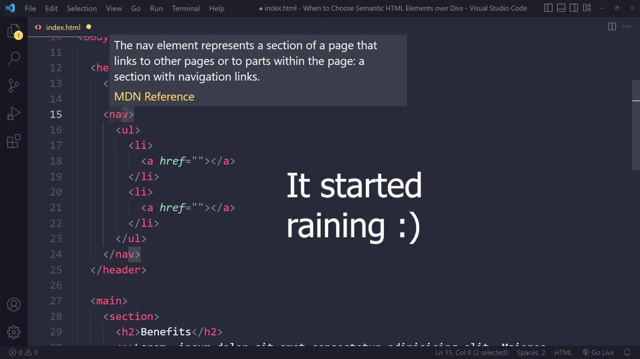 these out to get the laugh out of it. i've also preparedść about the women um the article tags that. that structure again, except now you wouldn't use the nav, so nav is typically more common in the header, because this is actually meant, as you know, a really important set of navigational links or 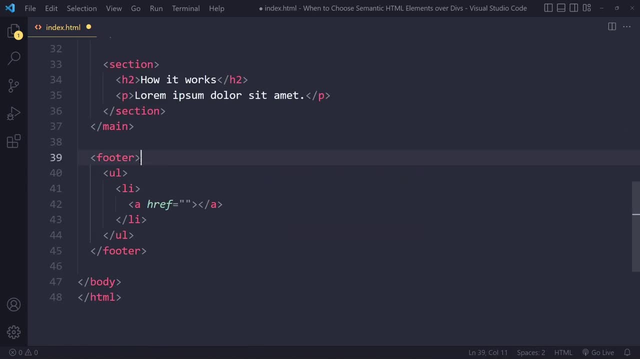 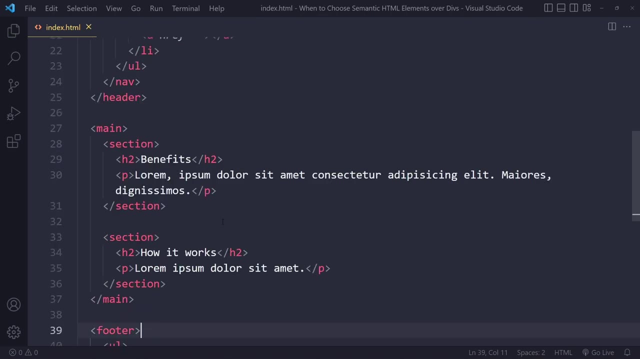 you know, navigational section. if it's really important, this probably shouldn't be in the footer right, so here you wouldn't see the nav tag right. so this is a really common, you know, semantic setup that you would see. and now we're going to look at some actual websites. 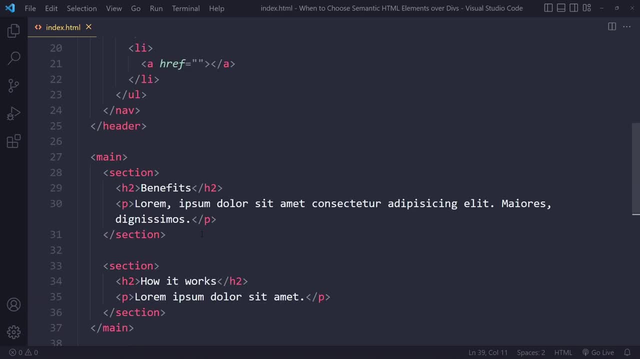 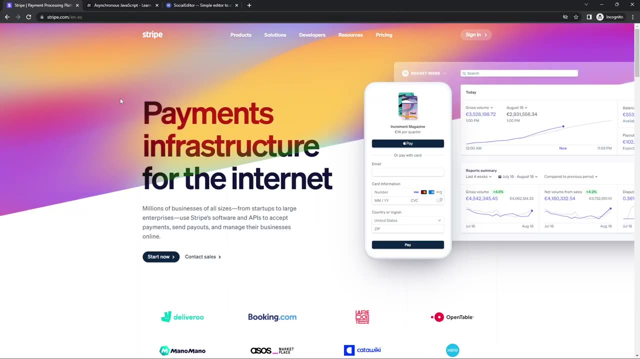 to see how they've done it, and i'll show you some of some examples for those more rare tags as well, like article and aside. all right, so this is the stripe website, but honestly i could have picked any landing page, because they're they're all quite similar. so we can inspect here and we can see how. 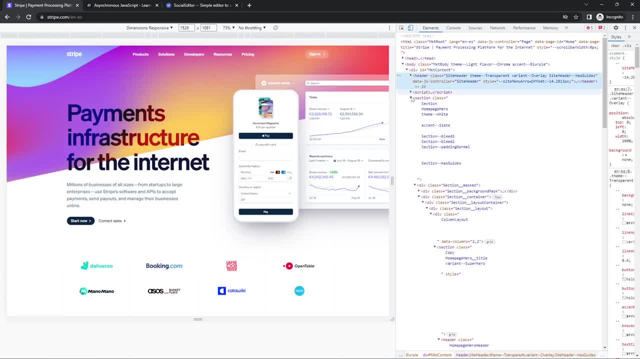 they've marked up their html. so in the at the top, we indeed see a header here, right? so here they have a logo, they have a bunch of important links and they have this sign in button, right, so that's a header for them, and they have a bunch of divs in here. 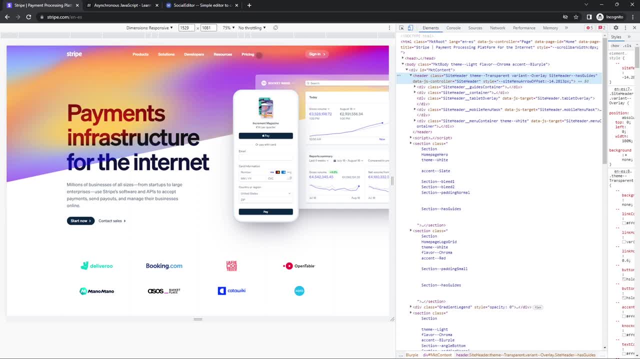 right, so that's a header for them and they have a bunch of divs in here. right, so that's a header for them and they have a bunch of divs in here, in here, because sometimes you need to use a div simply for stylistic purposes. let's see if we 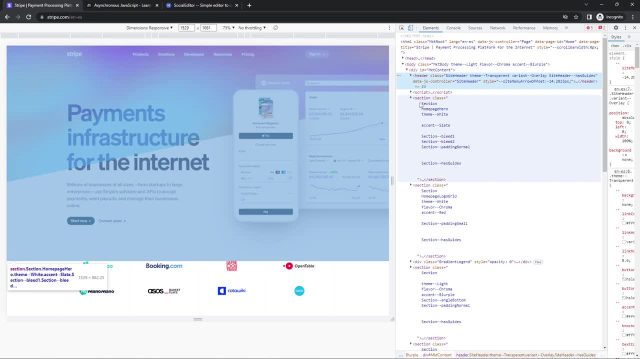 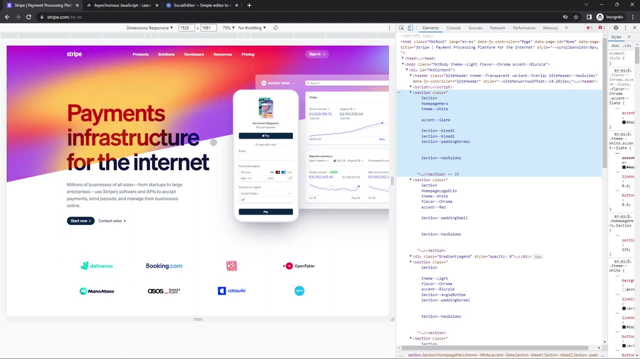 can find a good example here. doesn't look like it. maybe we'll find a good example of that later, but here we have a section. so this is what they call the, the hero section. right, really, the the the thing you look at first when you, when you come to the website. this is a section because all of this 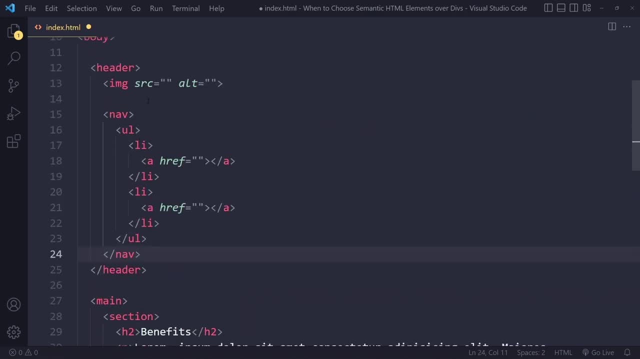 You wouldn't use the nav, So nav is typically more common in the header, because this is actually meant, as you know, a really important set of navigational links or, you know, navigational section. If it's really important, this probably shouldn't be in the footer. 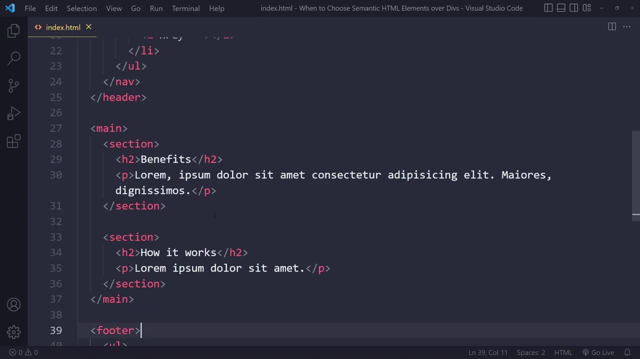 So here you wouldn't see the nav tag. So this is a really common, you know, semantic setup that you would see. And now we're going to look at some actual websites to see how they've done it And I'll show you some examples. 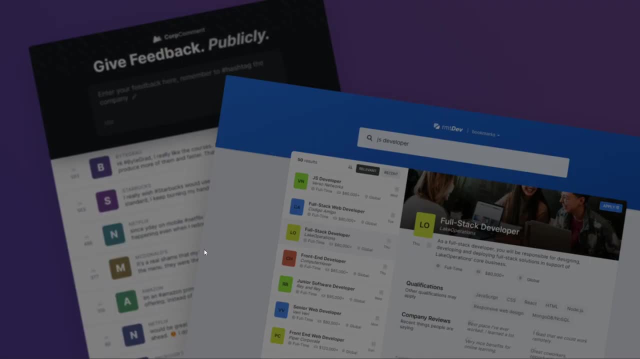 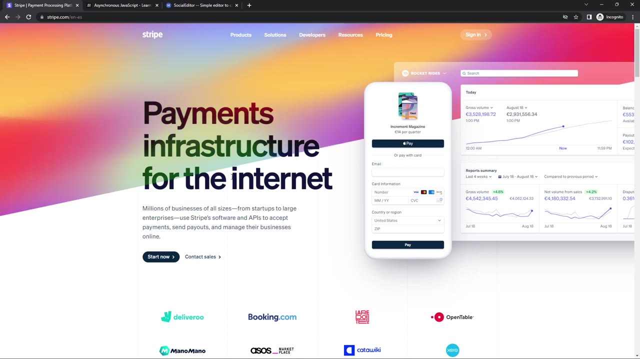 for those more rare tags as well, like article and aside. All right, so this is the Stripe website, but honestly I could have picked any landing page because they're all quite similar. So we can inspect here and we can see how they've marked up their HTML. 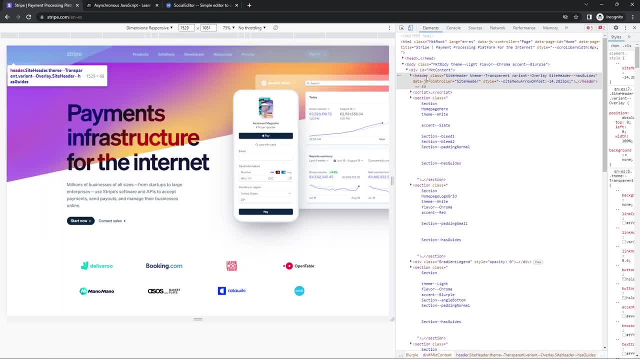 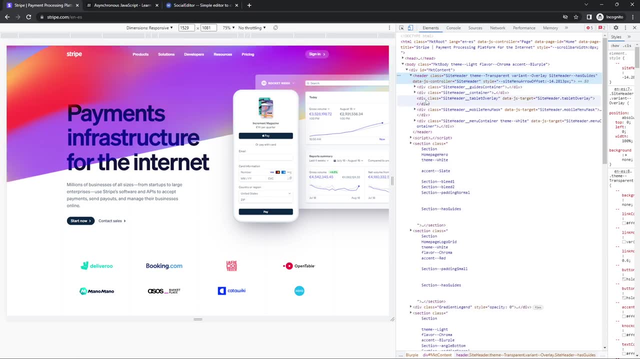 So at the top we indeed see a header here right. So here they have a logo, they have a bunch of important links and they have this sign in button right, So that's a header for them. They have a bunch of divs in here. 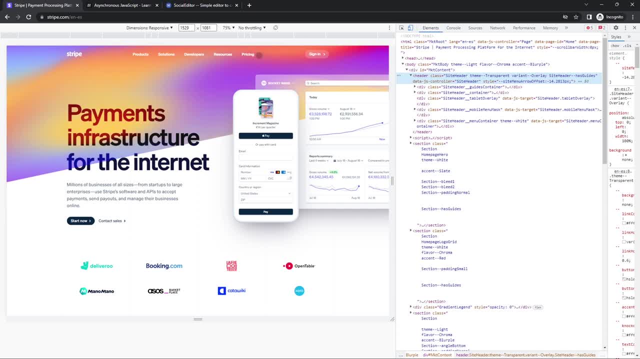 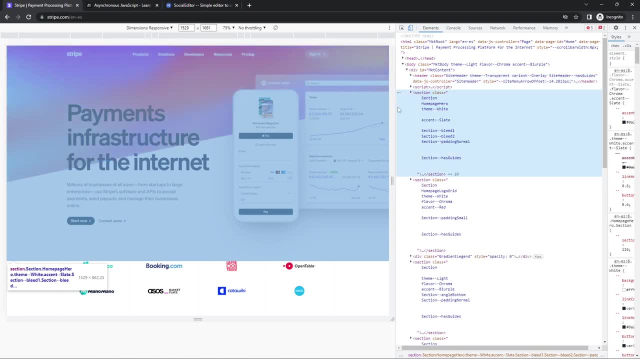 because sometimes you need to use a div simply for stylistic purposes. Let's see if we can find a good example here. It doesn't look like it. Maybe we'll find a good example of that later, But here we have a section. 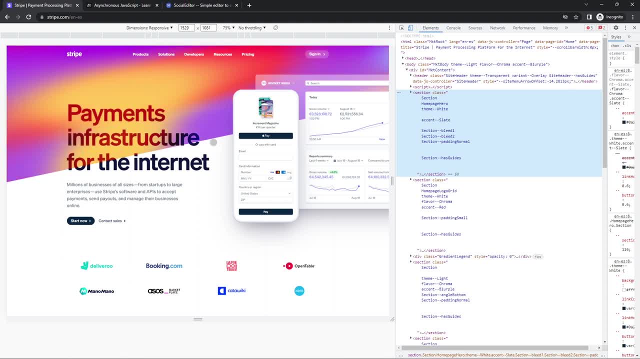 So this is what they call the hero section, right? Really, the thing you look at first when you come to the website. This is a section because all of this is related to each other. It's like a way to introduce their company or their product. 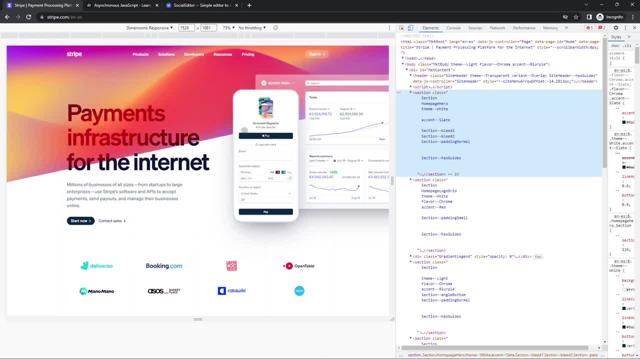 It's all related to each other. this heading and this text and this graphic, It all has the same semantic purpose and that's why it should be a section and not just a div right. So if it's a div, it would not be related to each other. 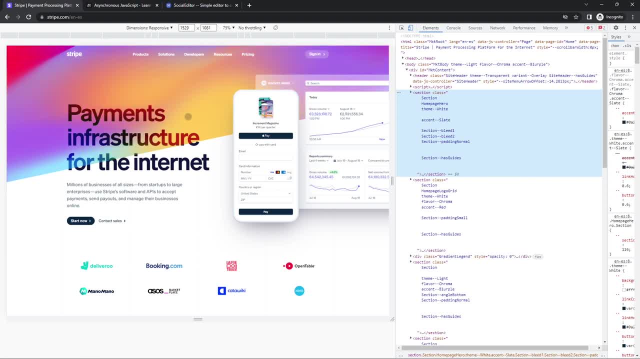 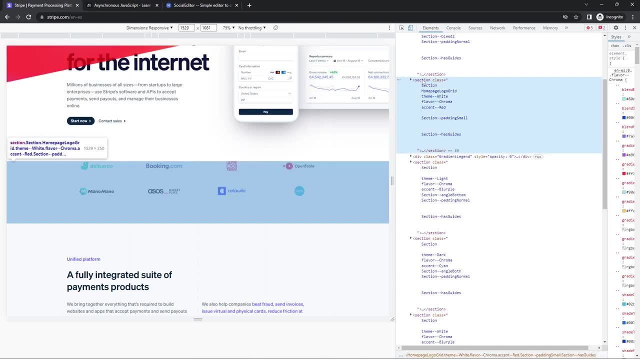 and you would only need some kind of element just for layout purposes. from stylistic purposes, you would use a div right. Then we get to this section here And let's see. So they used a section tag again And this is actually just a bunch of images actually, right? 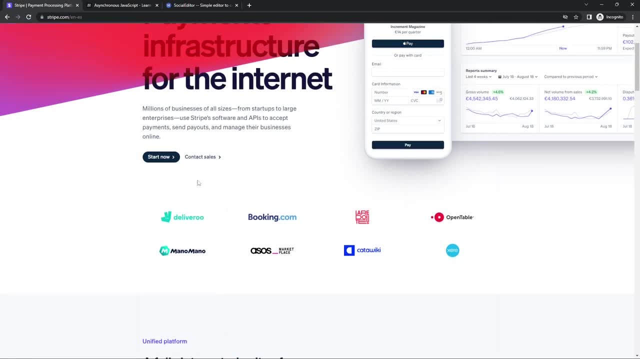 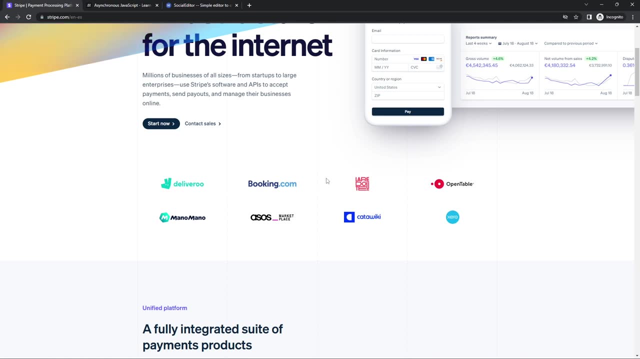 These images. well, what it represents is the type of companies that use. this is like credentials for them, And because each image here belongs to that same semantic purpose, they all should be in a section tag and not in a div right. 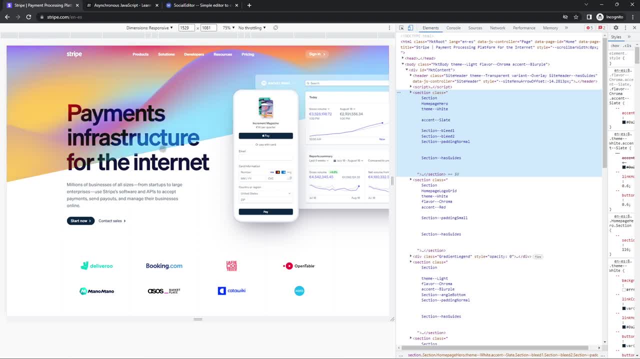 is related to each other. it's like a way to introduce their company or their product. it's all related to each other. this heading and this text and this, this graphic, it's all, uh, it all has the same semantic purpose and that's why it should be a section and not just a div right. so if it, 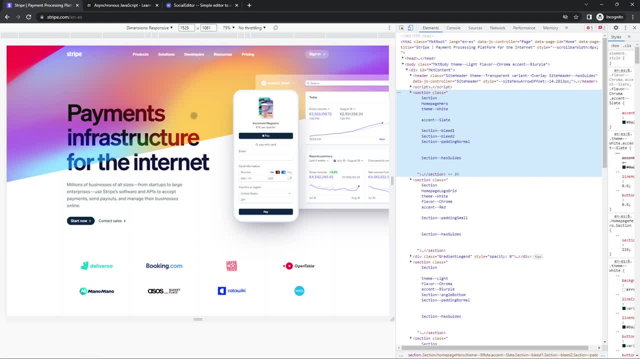 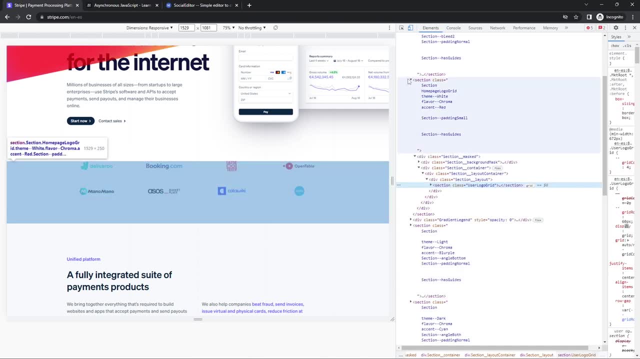 would not be related to each other and you would only need some kind of element just for layout purposes, from stylistic purposes, you would use a div, right. then we get to this section here and let's see. so they used a section tag again and this is actually just a bunch of images actually. 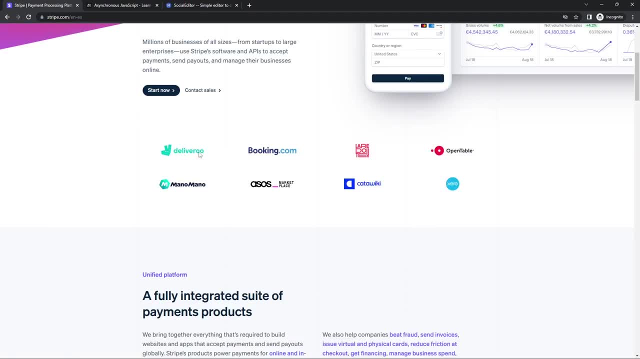 right these images? well, what? what it represents is the type of companies that you're going to be using for your business, and you're going to be using them for your business use, as this is like credentials for them, and because each image here belongs to that same. 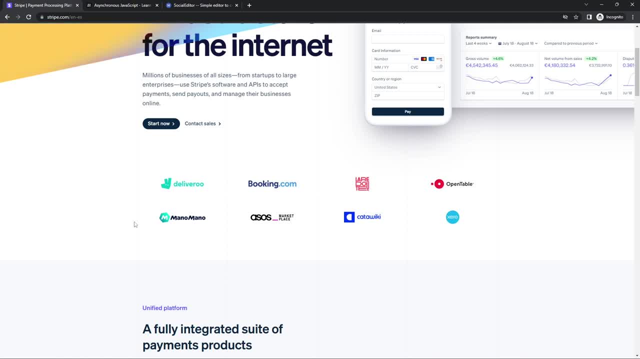 semantic purpose it. they all should be in a section tag and not in a div, because a section means that the content in there is related to each other. it has the same semantic purpose. so it's better to use the uh section tag. now, why not use the article tag here? well, article tag. 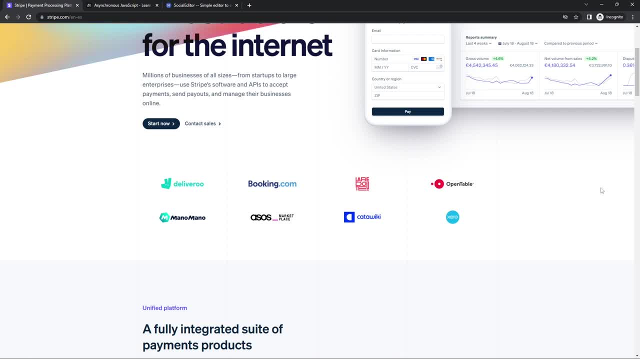 means that i should be able to pull this out of here, place it somewhere else, and it would still have the same meaning or it would still be clear what it means. but if i would take these images out of here and i would put it somewhere else on. 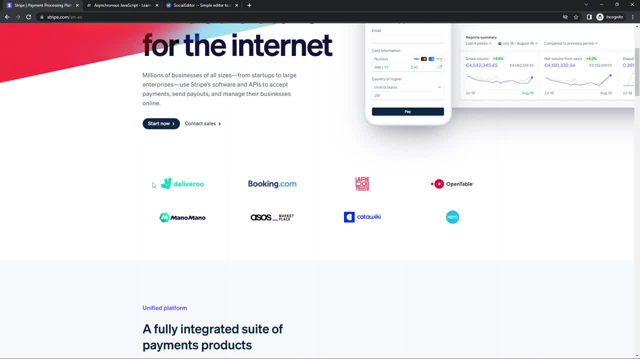 a different website or somewhere else. it would just be a you know collection of images. it wouldn't mean anything. it wouldn't mean the same as it means here, which is that these companies use stripe right. so this only makes sense in the context of the stripe website and therefore this: 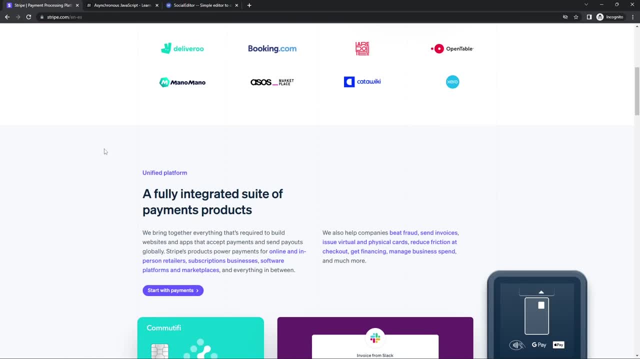 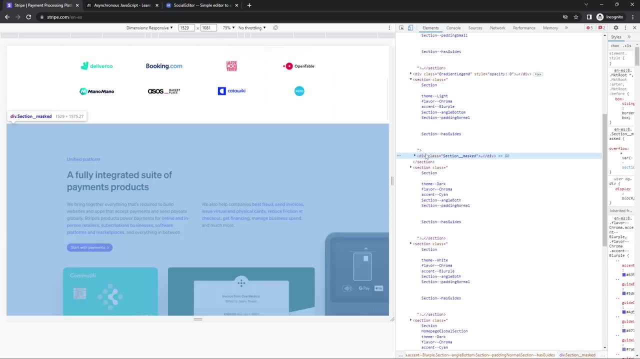 is not the article tag but a section tag. all right, so then if we go down you're gonna see a bunch of other sections they have that showcase why people should use right. so they want to convince the viewer to to use stripe. so here let's see this section. it has to do with 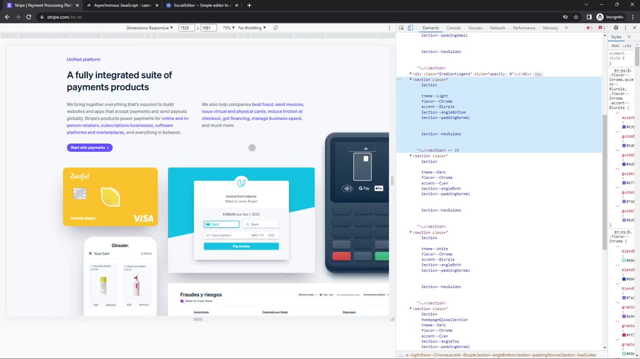 an overview of their product, and it's a section tag, because all of this in here is related to the, to it, to a, an overall semantic purpose, right? so this heading is not some standalone, random piece of text, right it's? it's a heading that describes everything else that's also part of 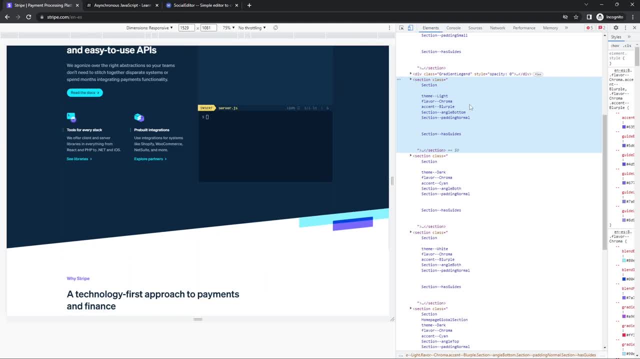 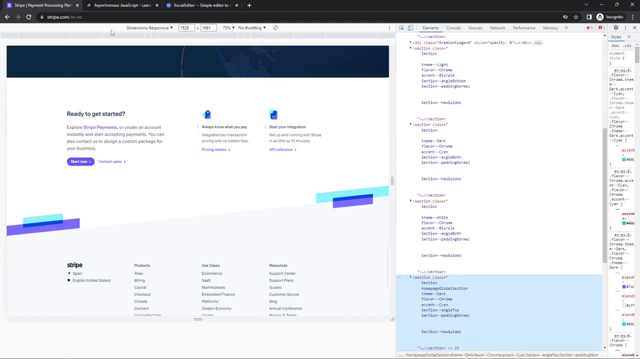 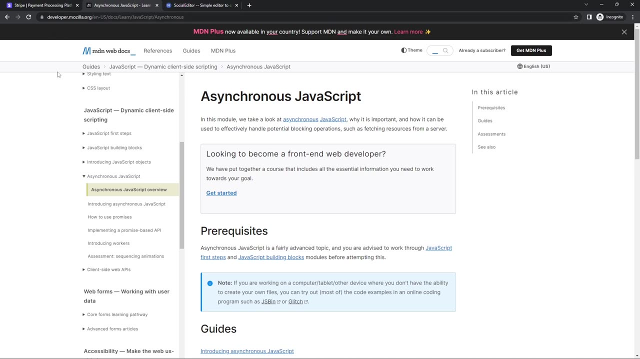 this, and so it's all related to each other, right? that's really what it comes down to with section versus div, right? so this is a section, this is a section, and usually it's quite easy to identify two or more of how you deal with it. 먼저, in juno degree right, say, let me show you more the. 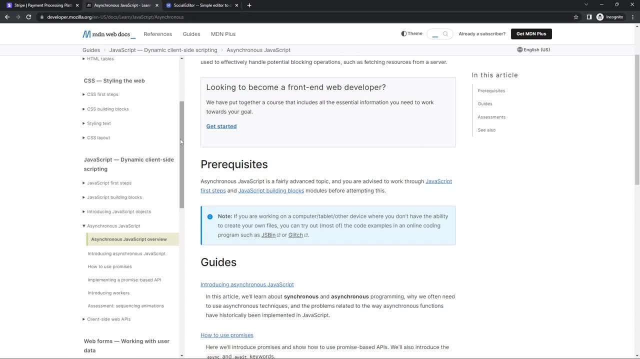 the syntax super 3.4 for juno 3, and then of course this is for theSerial, and then the a-centered page is really like it's kind of the main point right, because it's worth it a lot more than page for in Literacy in general. all in general they have content. 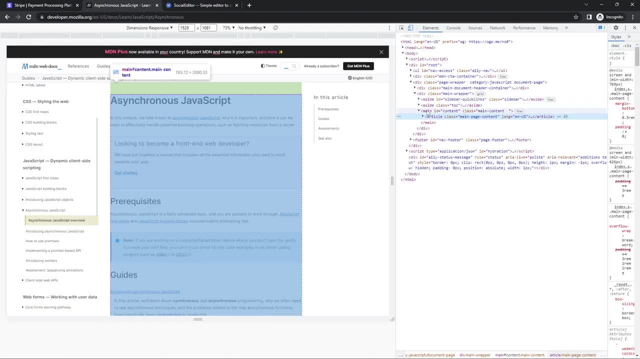 that以上 4 document, a clarification素 rd on page names in general also is great. you can see here. you see add师 a of the text that I made now writer background with that. so if you proof and i- lan of these landing pages. but this is a really typical example of sections versus div. all right now let's take a look at the mdn website. 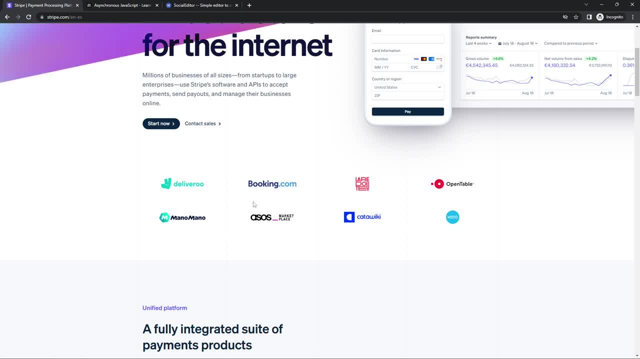 Because a section means that the content in there is related to each other. It has the same semantic purpose, So it's better to use the section tag. Now, why not use the article tag here? Well, article tag means that I should be able to pull this out of here. 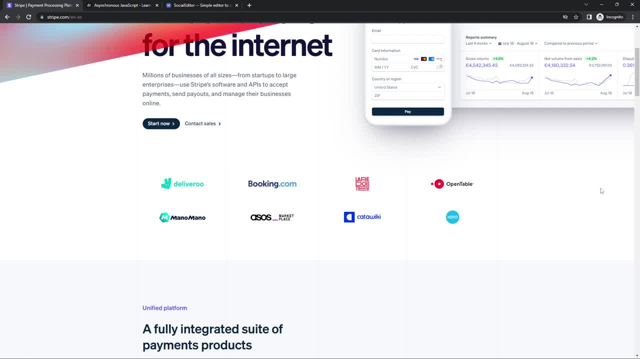 place it somewhere else and it would still have the same meaning or it would still be clear what it means. But if I would take these images out of here and I would put it somewhere else, on a different website or somewhere else, it would just be a collection of images. 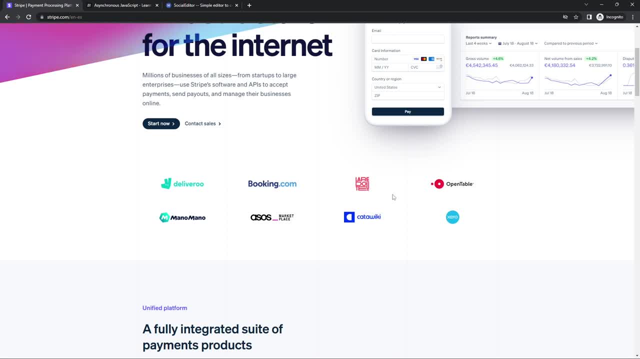 It wouldn't mean anything. It wouldn't mean the same as it means here, which is that these companies use Stripe right. So this only makes sense in the context of the Stripe website And therefore this is not the article tag. 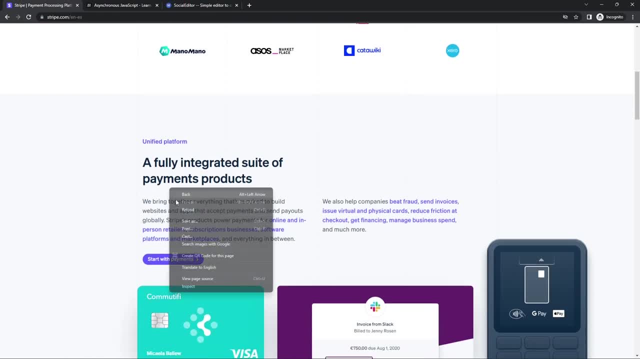 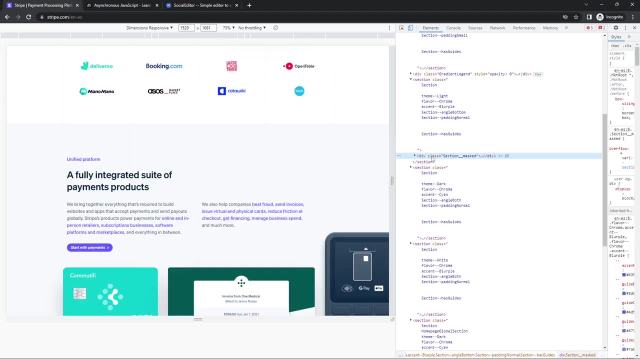 but a section tag, All right. so then if we go down you're going to see a bunch of other sections. they have that showcase why people should use right. So they want to convince the viewer to use Stripe. So here let's see this section. 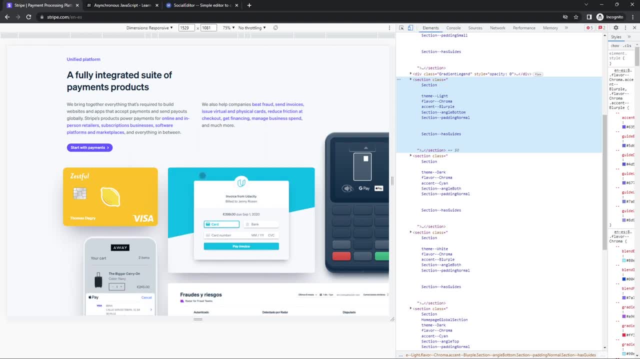 It has to do with an overview of their product And it's a section tag, because all of this in here is related to the, to an overall semantic purpose, right? So this heading is not some stand alone random piece of text, right? 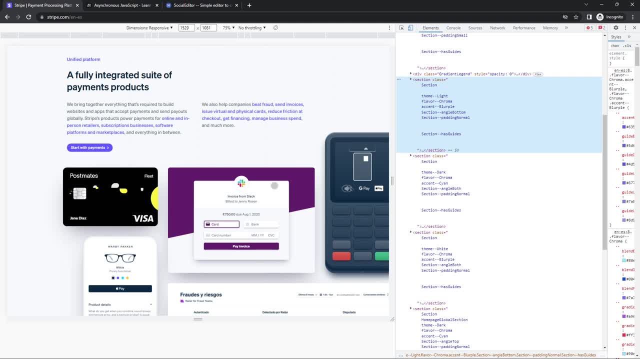 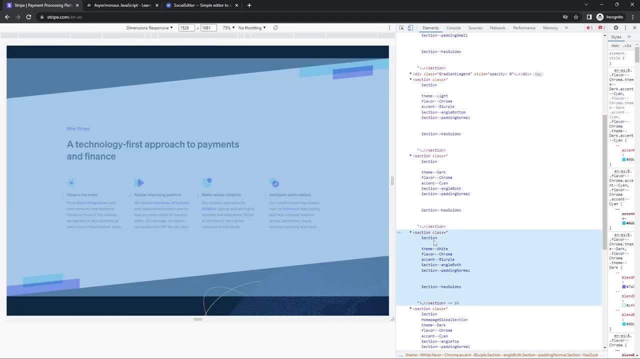 It's a heading that describes everything else. that's also part of this, And so it's all related to each other, right? That's really what it comes down to, with section versus div, right? So this is a section, this is a section. 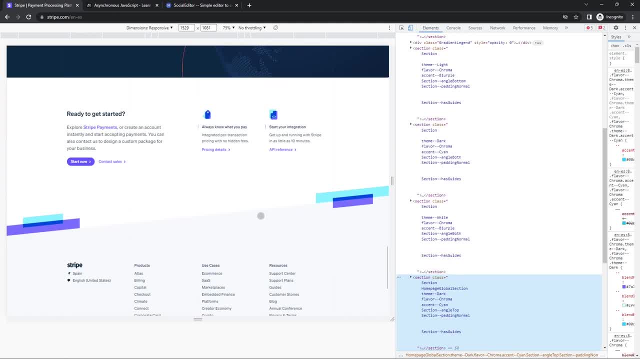 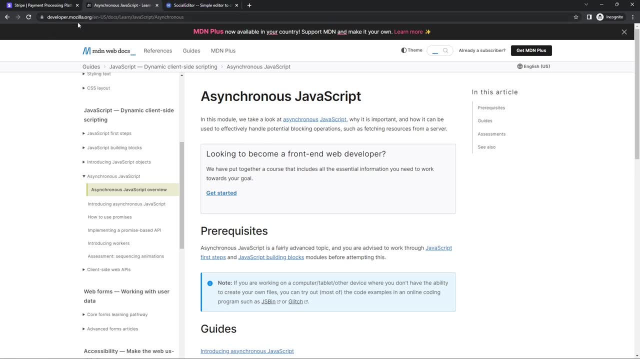 And usually it's quite easy to identify them on these landing pages. but this is a really typical example of sections versus div. All right, now let's take a look at the MDN website developermozillaorg. So if you go to one of their 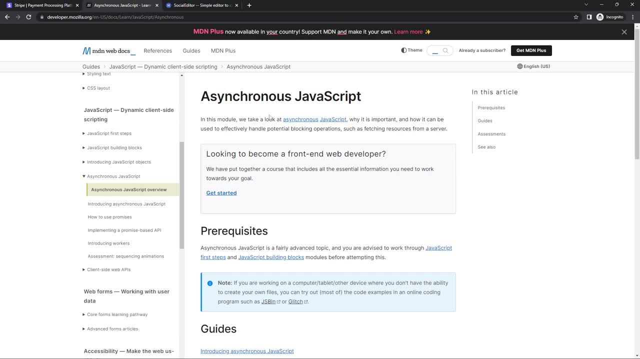 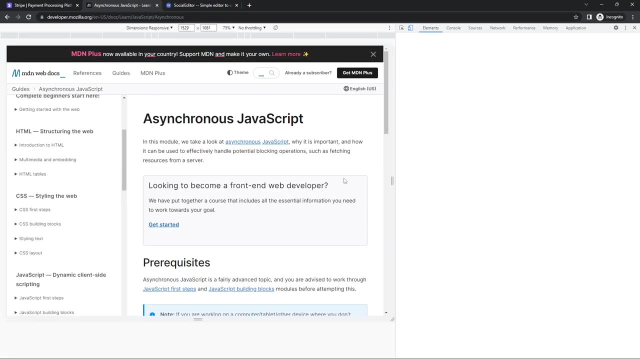 their articles. you can see that we have the actual content. We have some header on the top and then we also have this sort of sidebar. So let's see how they have marked this up. So here we can see this is the main content. 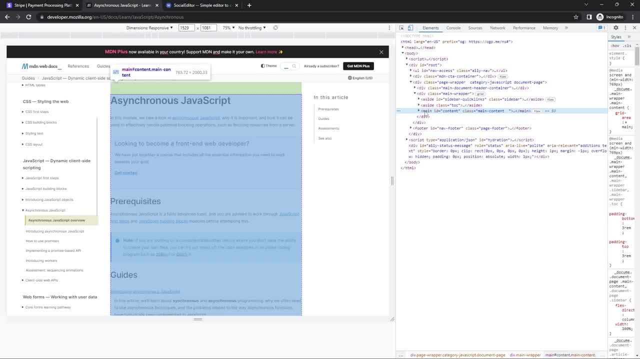 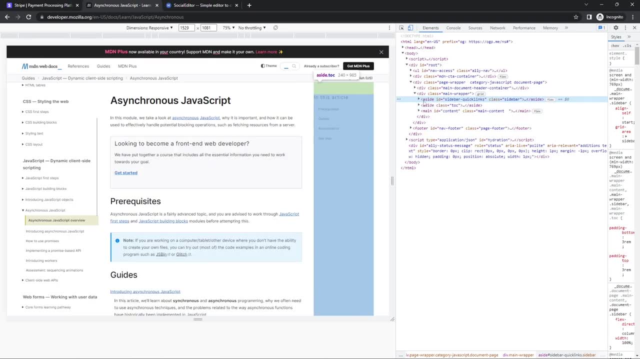 You're only gonna have one main tag on your page because it's for the most dominant content on the page And they've used an aside tag for this sidebar here, right, And actually you could make the argument that the aside never should be in the main. 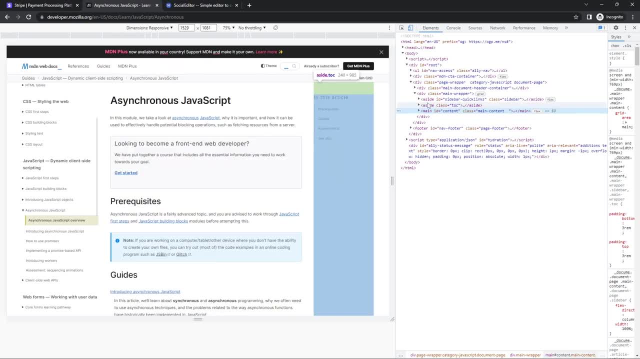 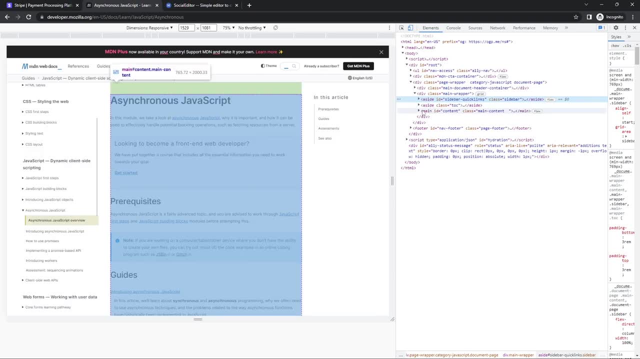 developermodeclaorg. so if you go to one of their uh articles, you can see that we have the actual content because it's for the most dominant content on the page and they've used an aside tag for this sidebar here. right, and actually you could make the argument that the aside never should be in the 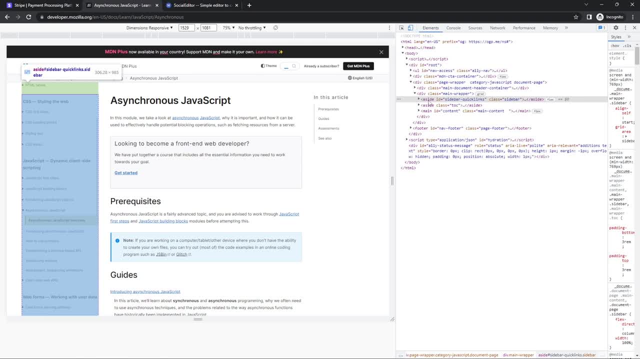 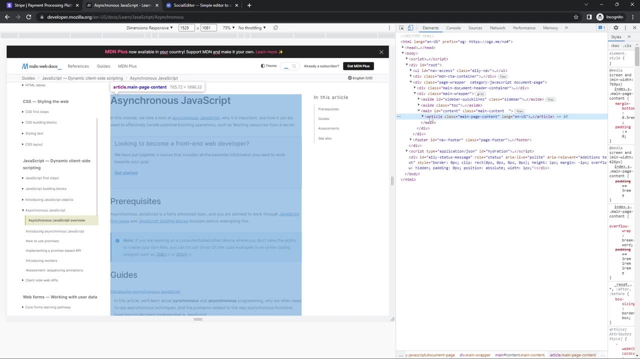 main because it's not really part of the dominant content, right, so you could make that argument. and then in the main we see an actual article tag here. so here they actually chose article instead of section, so article is actually a bit more like there's an additional requirement. that's how you. 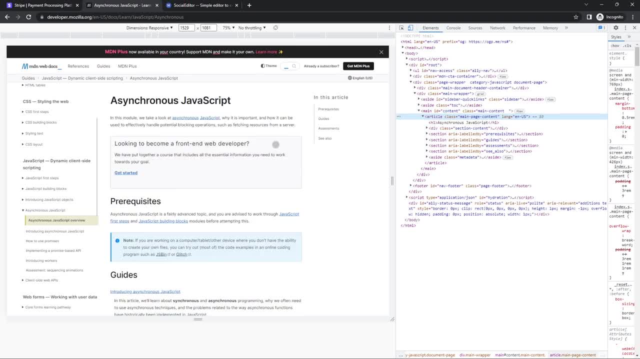 can think of it. so section just means that everything in there is related to each other or it has the same semantic purpose with article. the same has to be true. but i also need to be able to take this out of here and put it somewhere else and it should still make sense and that's actually. 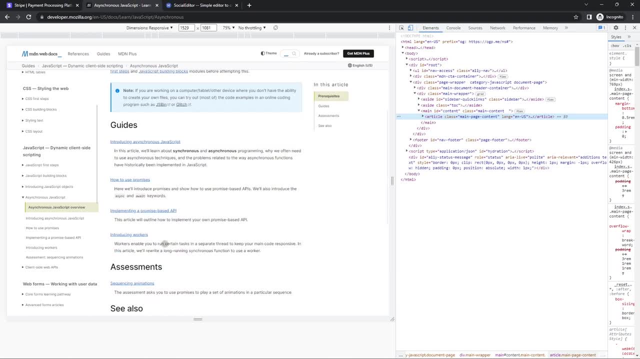 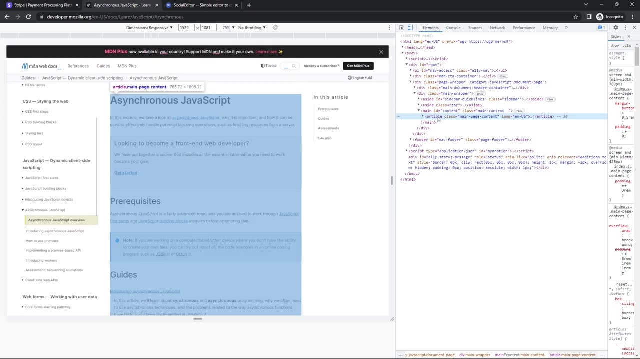 the case here. i could take out this, all of this text here. you could put it somewhere else, but it would. it would still be the same, it would still have the same value, essentially right. so it would still be clear what it is and therefore it should be an article tag. another example would be if, for 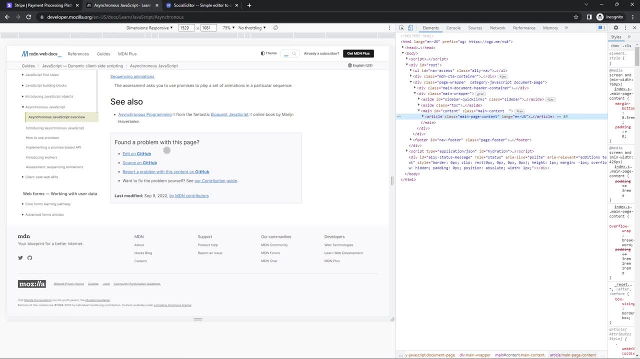 example, they had some kind of job posting here, right, maybe they they have some kind of um you know- job post. that would also be a good candidate for an article tag, because i could take the job post out of this website. i could put that somewhere else, maybe on like um, a jobs website, and it would still make sense there, right, i could put. 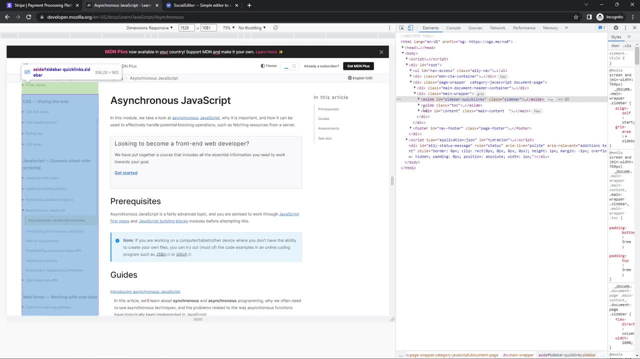 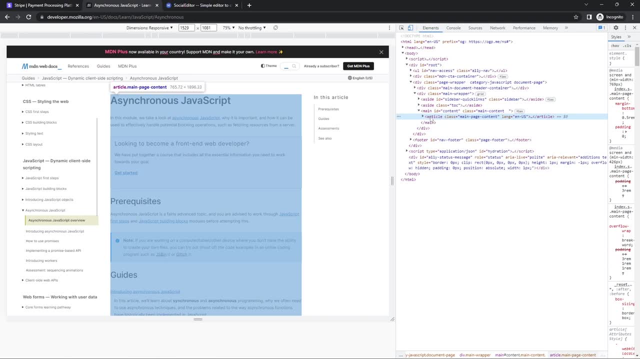 because it's not really part of the dominant content right. So you could make that argument And then in the main we see an actual article tag here. So here they actually chose article instead of section, So article is actually a bit more. 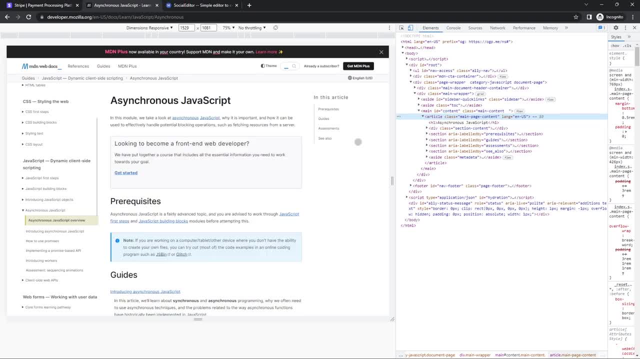 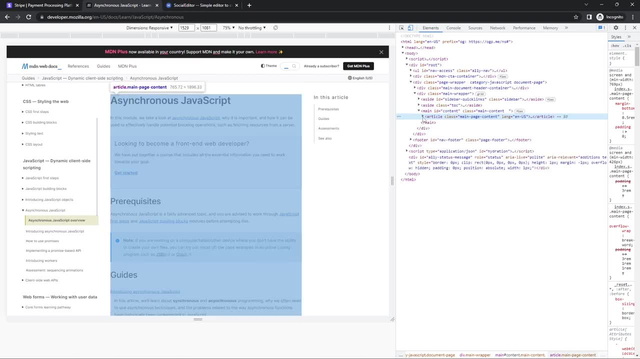 like there's an additional requirement. That's how you can think of it. So section just means that everything in there is related to each other or it has the same semantic purpose With article. the same has to be true, but I also need to be able to take this out of here. 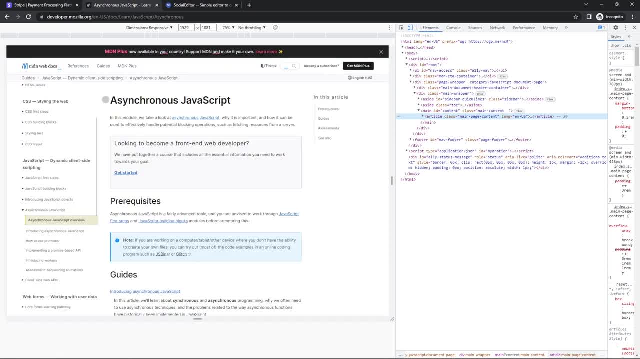 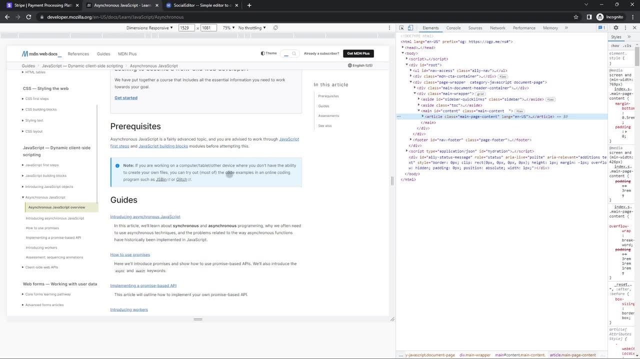 and put it somewhere else, and it should still make sense, And that's actually the case here. I could take out this, all of this text here. You could put it somewhere else, but it would still be the same. It would still have the same value, essentially right. 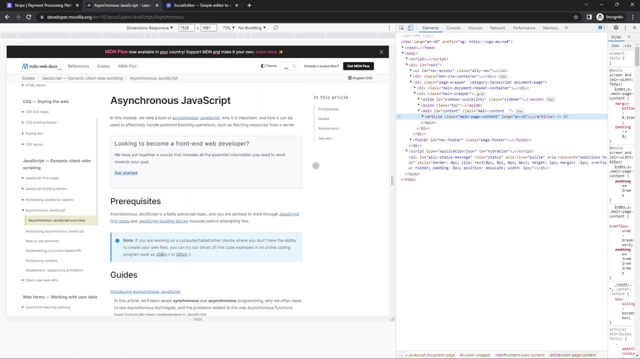 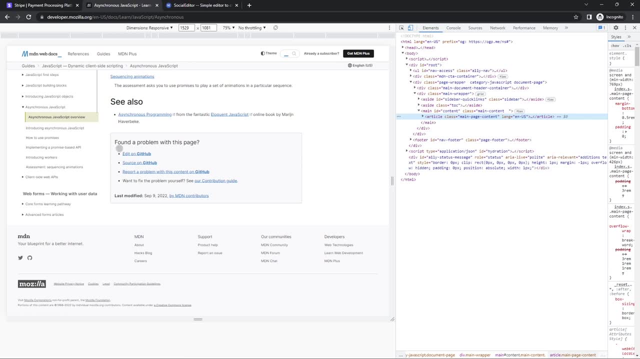 So it would still be clear what it is And therefore it should be an article tag. Another example would be if, for example, they had some kind of job posting here, right, Maybe they have some kind of- you know- job post. 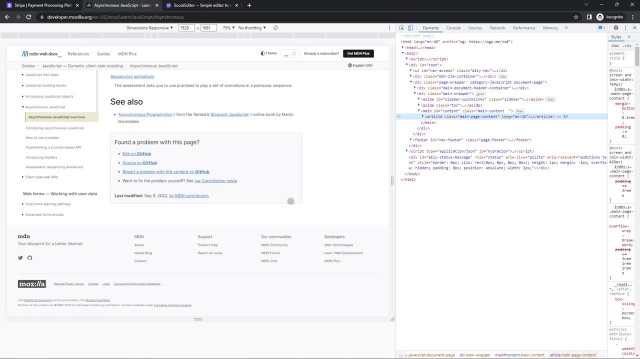 That would also be a good candidate for an article tag, because I could take the job post out of this website. I could put that somewhere else, maybe on like a jobs website, and it would still make sense there, right, I could put it on any other website. 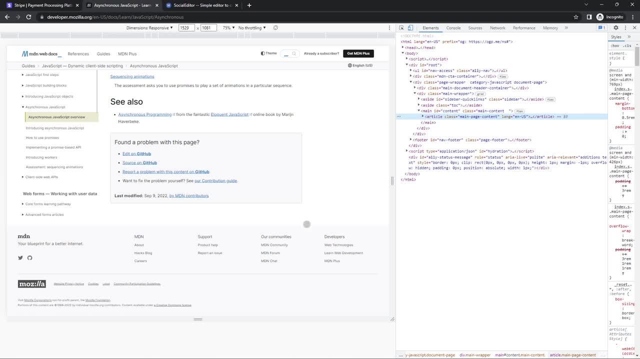 and it would still make sense. That article tag is self-contained, It explains itself. You can look at it, you can read it, you can consume it, and it's clear what it is, what its purpose is, what it represents. 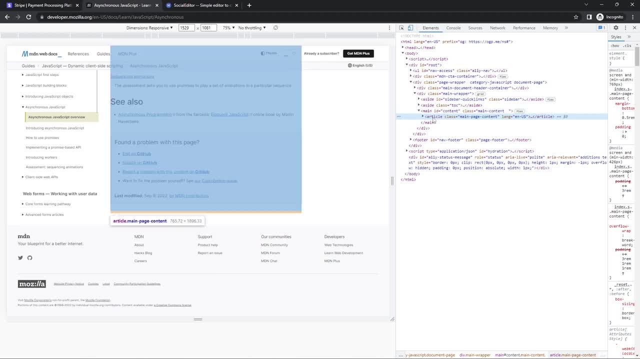 and therefore you want to use an article tag. Now, this is quite rare. The aside and article tags, you don't use them. You don't use it often. In most of your projects you're gonna use the section tag and a bunch of divs. 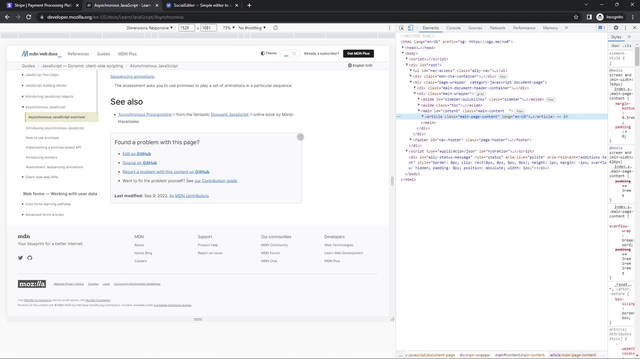 it on any other website and it would still make sense. that article tag is self-contained, it explains itself, it you can. you can look at it, you can read it, you can consume it, and it's clear what it is, what its purpose is, what it represents and therefore it's a good candidate for an article. 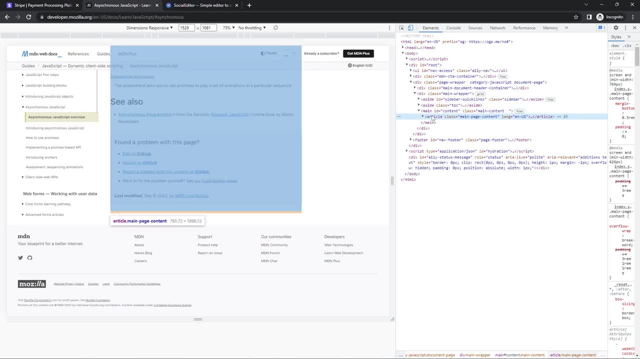 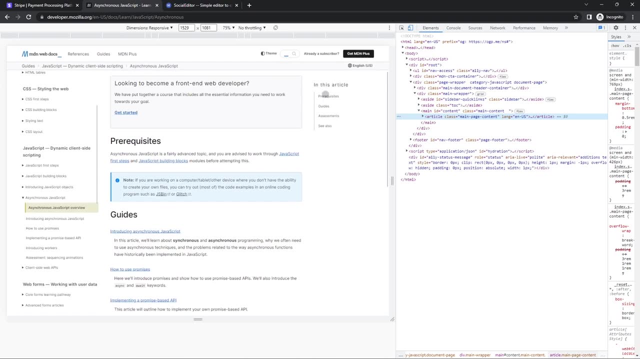 tag- now this is quite rare. the aside and article tags you don't use that much. you don't use it often in most of your projects you're going to use the section tag and a bunch of divs, okay, so here they also have some kind of navigation here. so this is maybe interesting to look at as well. so 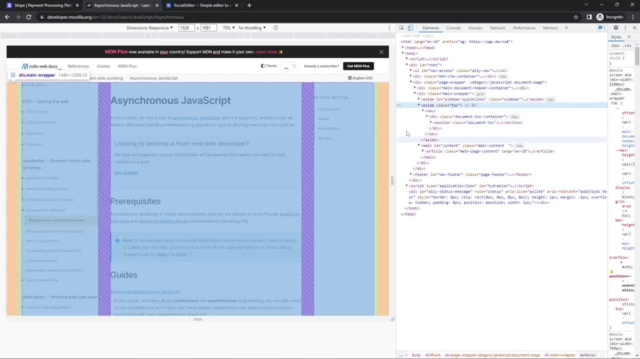 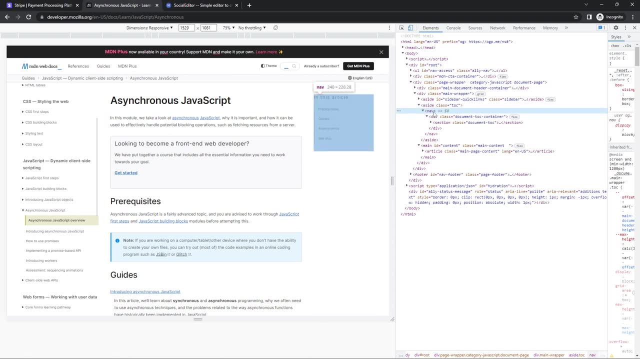 here they use the section for that. actually they use an aside for this overall piece and then they use a nav tag again, and that's right. so you're not only going to see a nav in the header, but also sometimes outside of there if it's an important set of navigation, which it is right. 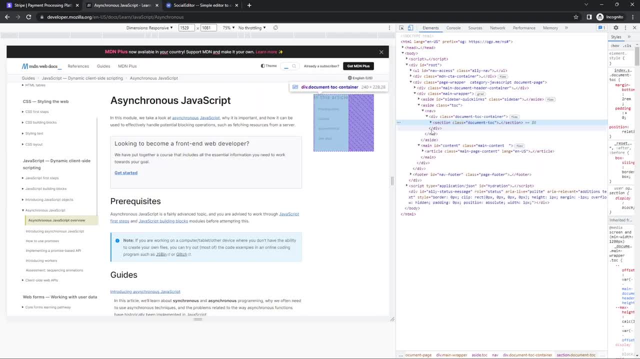 Okay, so here they also have some kind of navigation here, So this is maybe interesting Now to look at as well. So here they use the section for that. Actually they use an aside for this overall piece, and then they use a nav tag again. 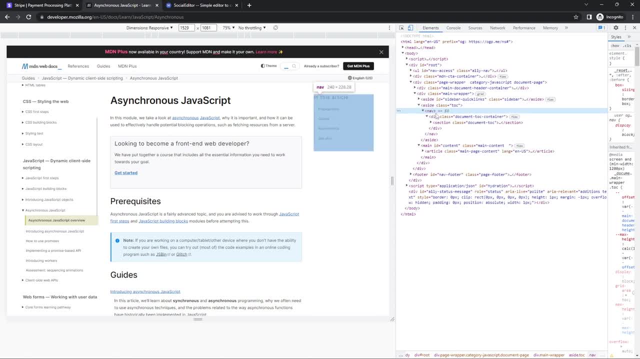 And that's right. So you're not only gonna see a nav in the header, but also sometimes outside of there, if it's an important set of navigation, which it is right. So this, like a table of contents, is an important piece of navigation. 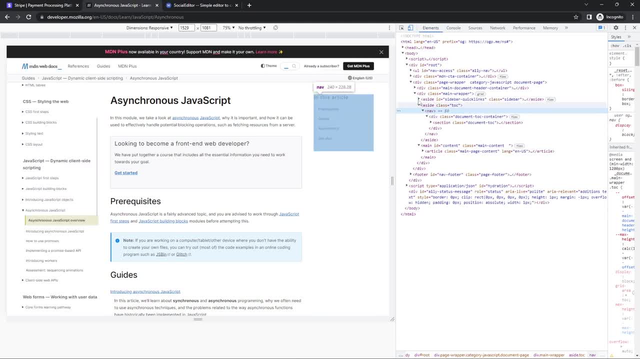 So you could opt for using the nav tag there. This all may seem a little bit confusing and overwhelming In practice. you know, if you didn't use nav here but you used just an UL perhaps, or maybe a section instead of an aside? 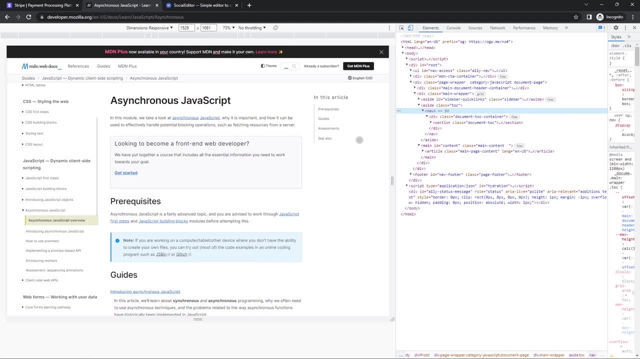 so this, like a table of contents, is an important uh piece of navigation, so you could opt for using the nav tag there. this all may seem a little bit confusing and overwhelming in practice. you know if you would if you didn't use nav here, but you used just an ul perhaps, or maybe a section instead. 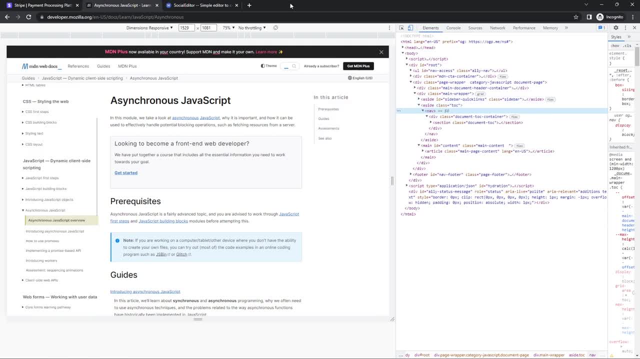 of an aside. all of that is generally fine in practice. um you know it, it doesn't matter that much for readability of your html. the search engines don't really care that much. i mean, they must be pretty adept at this point in time. so i think it's a good idea to use a nav tag. 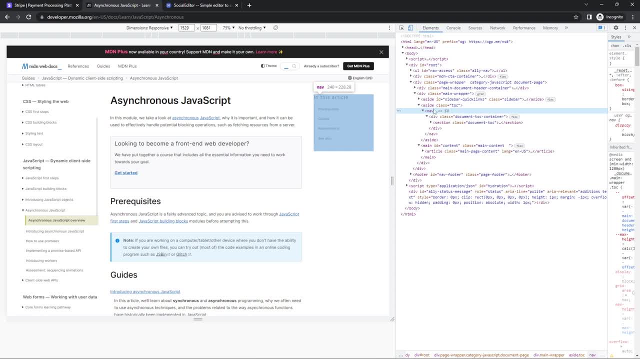 to dealing with with unstructured html, because most websites out there are quite unstructured, so all of this doesn't make that much sense. you know to to spend a lot of time and energy on, but you know, if you want to be precise about it, that's how you would do it. now i want to give you one example. 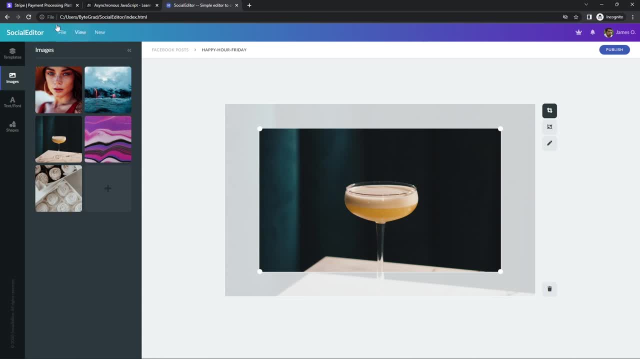 of where you would use the div instead of the section right, because now we've seen a couple of examples of where to use something else than div. so then, where should you use actually? where should you actually use divs? well, basically everywhere else. so here, for example, and this: 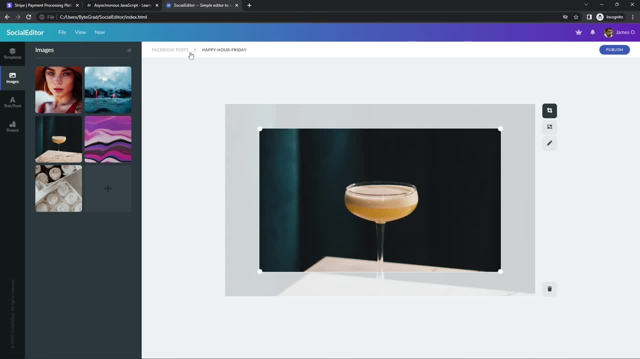 is one of my projects from my css course. here we have a bunch of like. we have some- well, these are breadcrumbs, and then we have some other button on the other side. now, this is not really related to each other, they're just stylistically speaking in the same white bar. 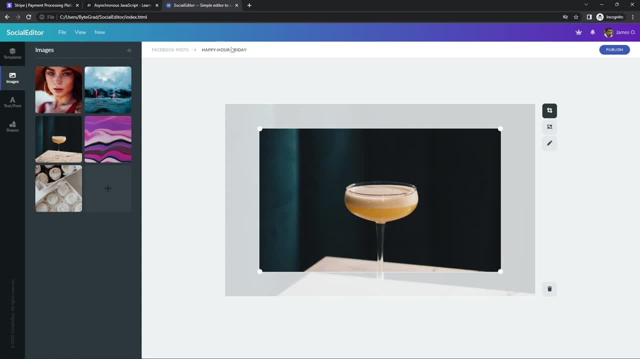 here, but they have different um purposes, right, they don't have, they're not. they don't belong to the same semantic purpose. but they are still stylistically in the same bar here and therefore you probably need some kind of element in your html to get the proper layout. so in that case, 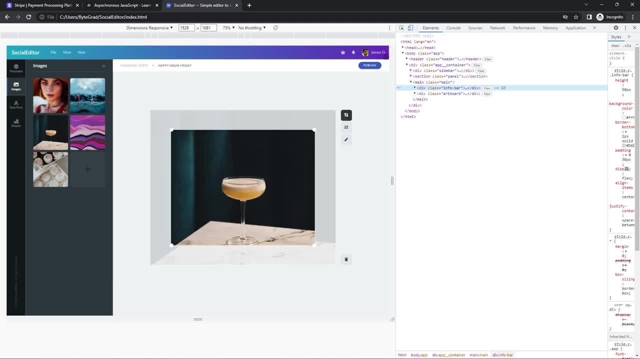 you want to use the div, actually right. so here there's some kind of info bar, but they're two different things. this is breadcrumbs- i used a section for that- because the text, the text in there, they all belong to the same uh well, overall semantic, uh goal and this is a button tag, but they are two completely different things. 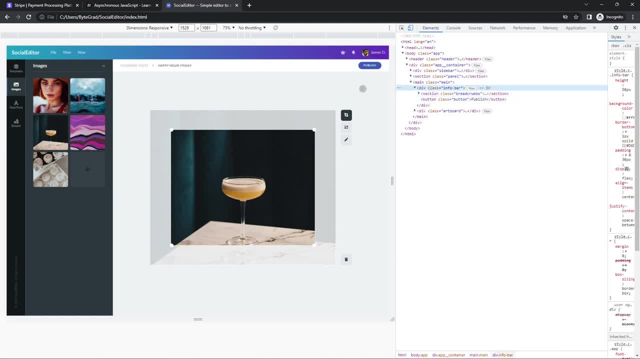 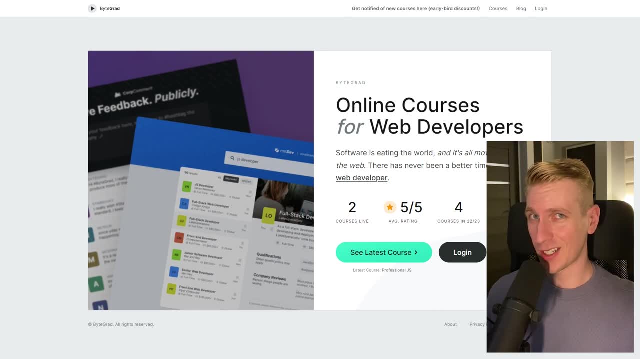 they don't have anything to do with each other, but i still needed some kind of element to get this layout right. so here i would. i would not use section, i would use a div. by the way, if this was helpful, i'd really appreciate it if you could like and subscribe. also check out my courses on css and 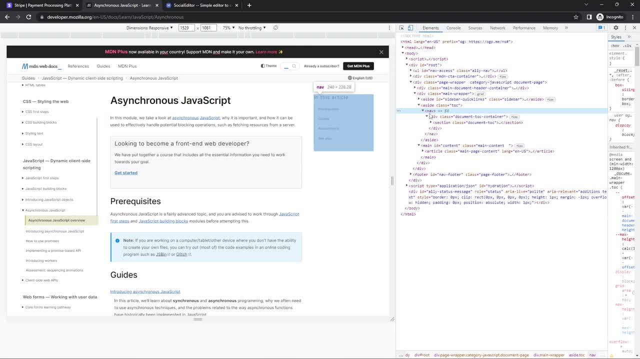 all of that is generally fine in practice. You know it doesn't matter that much for readability of your HTML. The search engines don't really care that much. I mean, they must be pretty adept at this point to dealing with unstructured HTML. 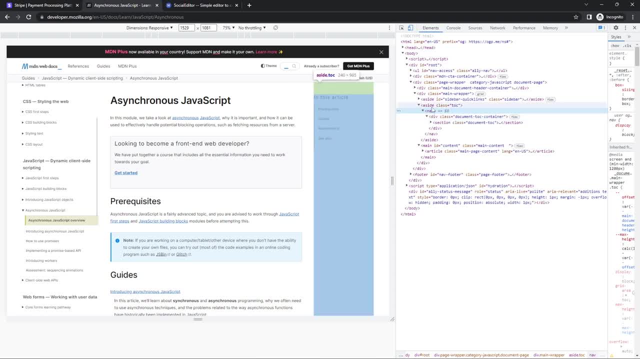 because most websites out there are quite unstructured, So all of this doesn't make that much sense. you know to spend a lot of time and energy on, but you know, if you wanna be precise about it, that's how you would do it. 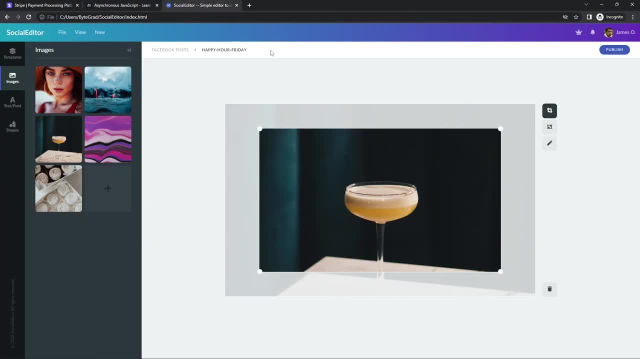 Now I wanna give you one example of where you would use the div instead of the section right, Because now we've seen a couple of examples of where to use something else than div. So then, where should you actually use divs? Well, basically everywhere else. 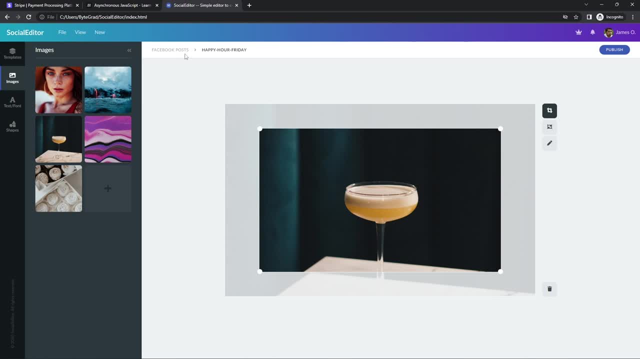 So here, for example- and this is one of my projects for my CSS course- here we have a bunch of like. we have some- well, these are breadcrumbs- and then we have some other button on the other side. Now, this is not really related to each other. 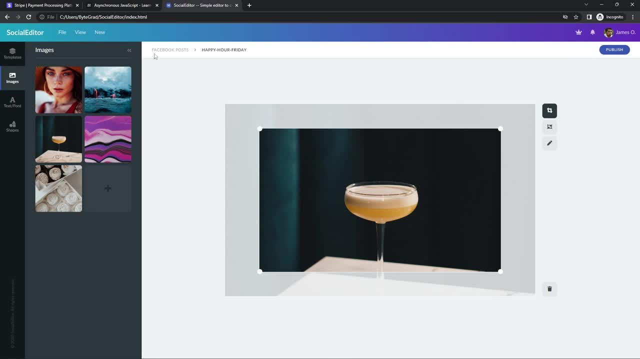 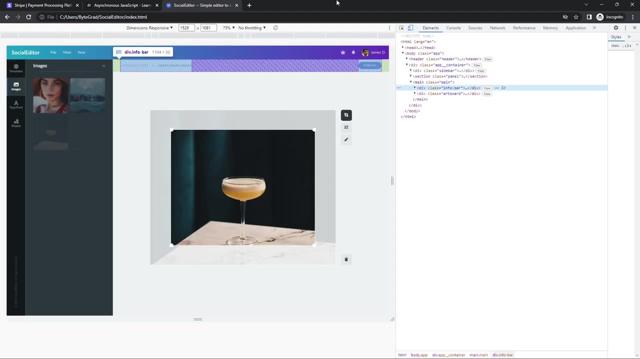 They're just stylistically speaking, in the same white bar here, but they have different, different purposes. right, They don't belong to the same semantic purpose, but they are still stylistically in the same bar here And therefore you probably need some kind of element. 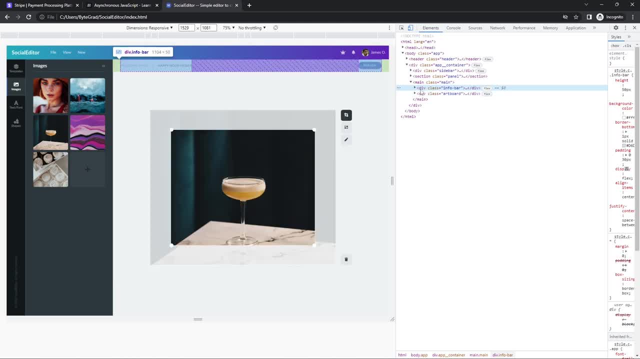 in your HTML to get the proper layout. So in that case you wanna use the div actually, right. So here there's some kind of info bar, but they're two different things. This is breadcrumbs. I use the section for that because the text in there 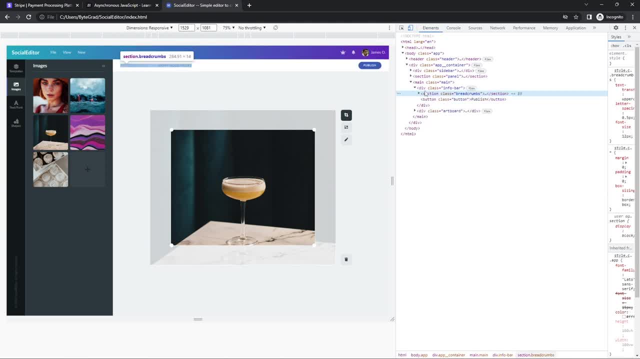 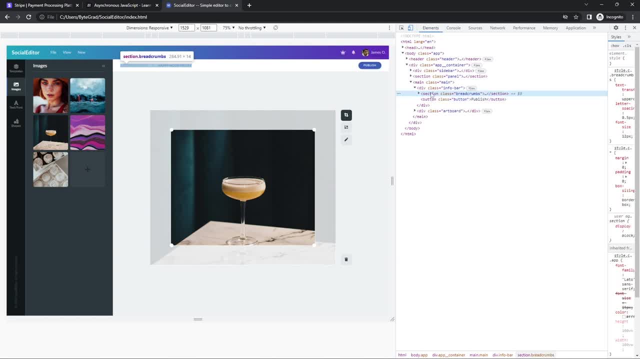 And this is a button type. But they are two completely different things, They don't have anything to do with each other. but I still needed some kind of element to get this layout right. So here I would not use section, I would use a div. 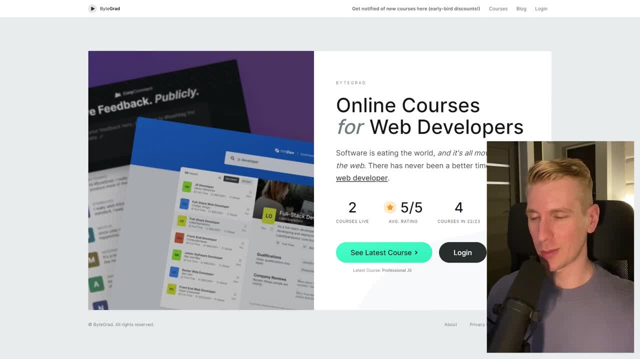 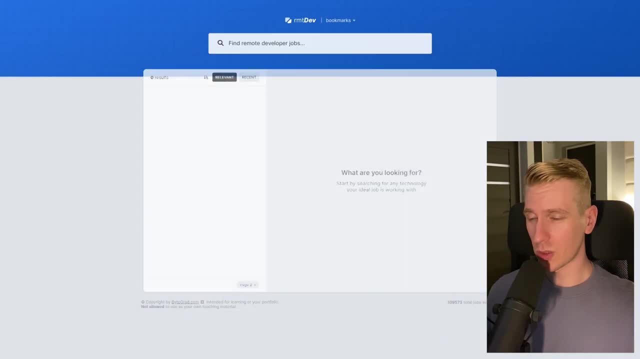 By the way, if this was helpful, I'd really appreciate it if you could like and subscribe. Also, check out my courses on CSS and JavaScript if you wanna take those skills to an advanced level, because in there we will build some beautiful real-world projects from scratch. 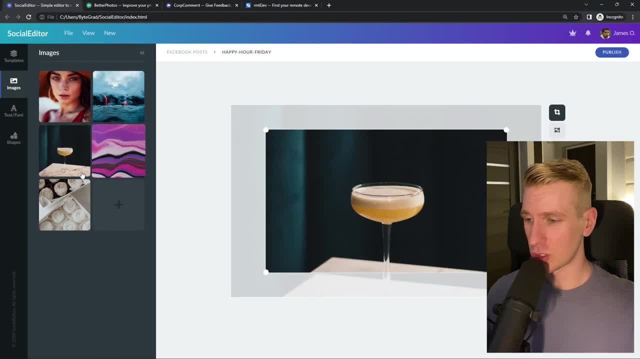 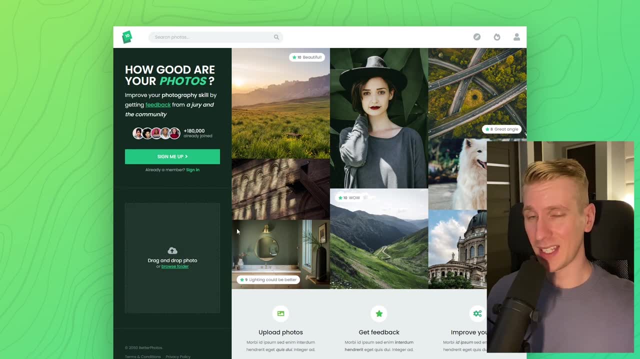 so you can see how everything fits together and really master CSS or JavaScript. And I will also release other courses soon like React and Nodejs. So if you wanna be doing that, be notified and make sure you are subscribed to the email newsletter. You can find the link in the description. Thanks for watching and I hope to see you soon. 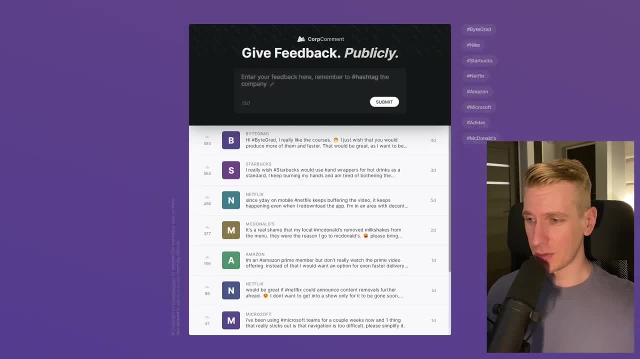 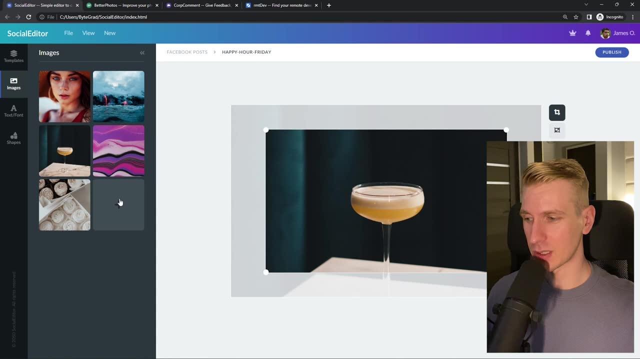 javascript if you want to take those skills to an advanced level, because in there we will build some beautiful real world projects from scratch so you can see how everything fits together and really master css or javascript. and i will also release other courses soon, like react and nodejs. so if you want to be notified, then make sure you are subscribed to the 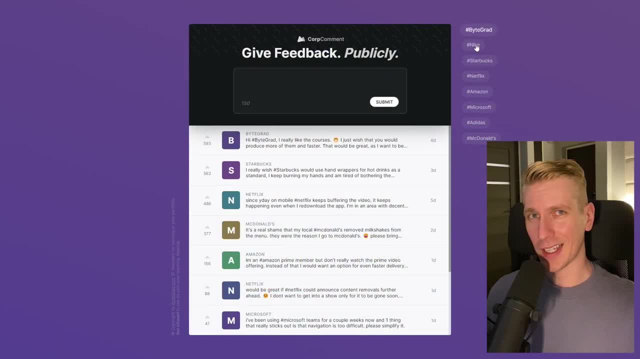 email newsletter. you can find the link in the description. thanks for watching and i hope to see soon. 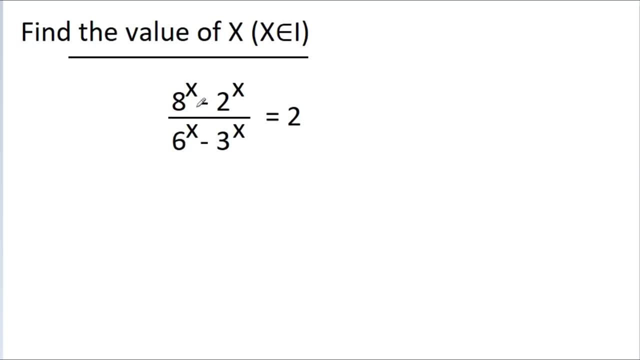 In this video we have given that 8 to the power, x minus 2 to the power, x by 6 to the power x minus 3 to the power, x is equal to 2.. And we have to find the value of x, where x belongs to integers. So here we have given that 8 to the power x minus 2 to the power. 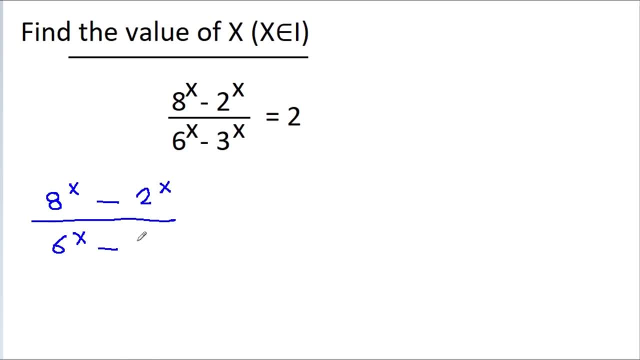 x by 6 to the power x minus 3 to the power x is equal to 2.. And now 8 is equal to 2 cube, So it will be 2 cube. power x minus 2 to the power x by 6 is equal to 2 into 3.. It is 2. 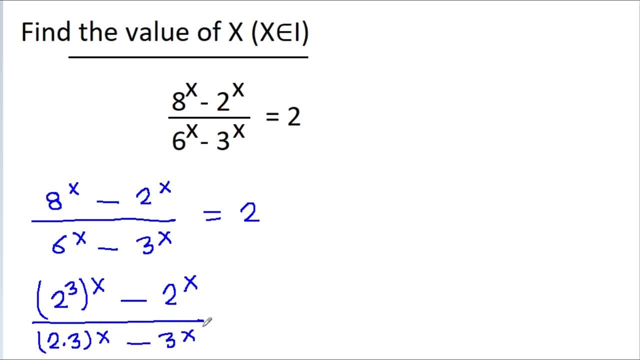 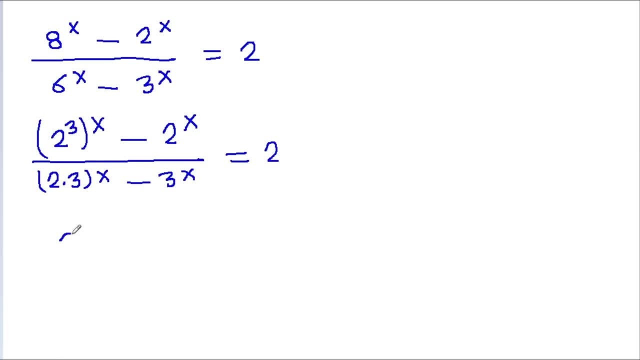 into 3, power x minus 3 to the power x is equal to 2.. And now 2 cube power x minus 3 will be 2 to the power. 3. x minus 2 to the power x by 2 into 3, power x will be 2 to the. 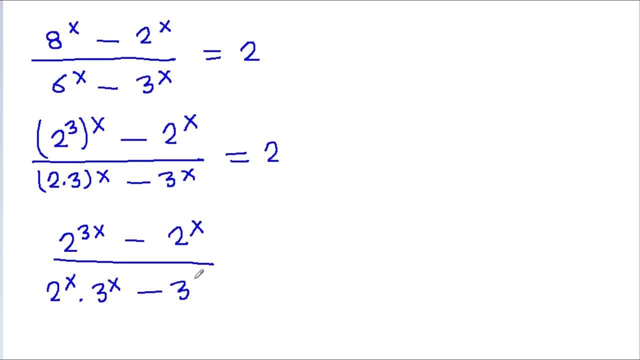 power x into 3 to the power x minus 3 to the power x is equal to 2.. And now, here, if we take 2 to the power x common, then we get 2 to the power 2 x minus 1.. And here, if we 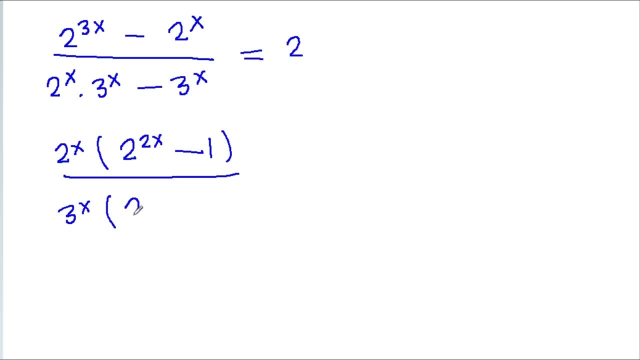 take 3 to the power 3, x minus 3 to the power x is equal to 2.. And now, if we take 2 to the power x common, then we get 2 to the power x minus 1 is equal to 2.. And now we know that.